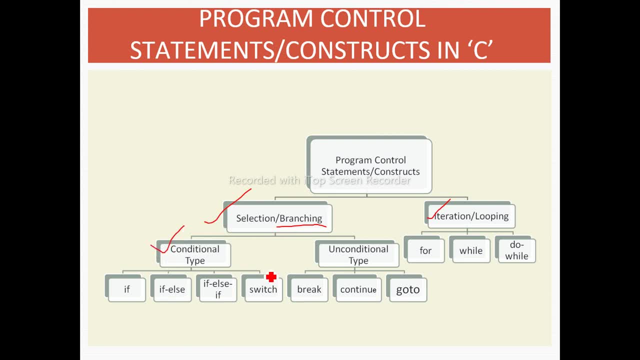 a selection branching. There are two types: conditional and unconditional. in the conditional we can give a condition to block of statement should get executed and in unconditional we can directly go to that particular statement or a block of statement to get executed. So this is the whole classification. 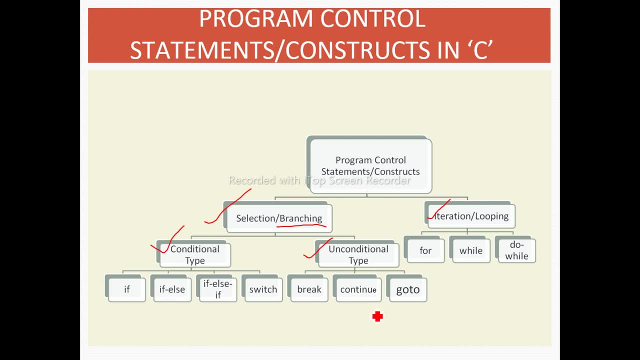 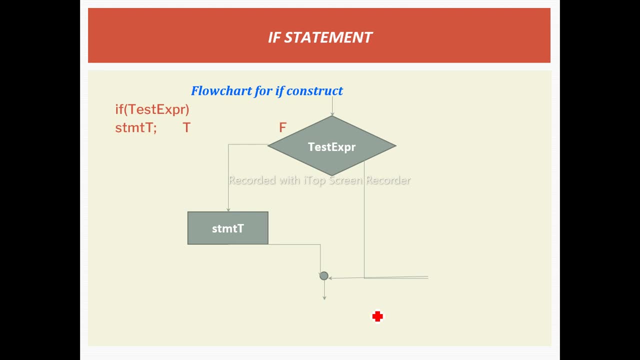 of branching or control statements. So firstly we will learn what is the conditional type of statement or block of statement. So this is the syntax is given for the if statement. In a if statement, firstly we need to give a condition. and if this condition becomes 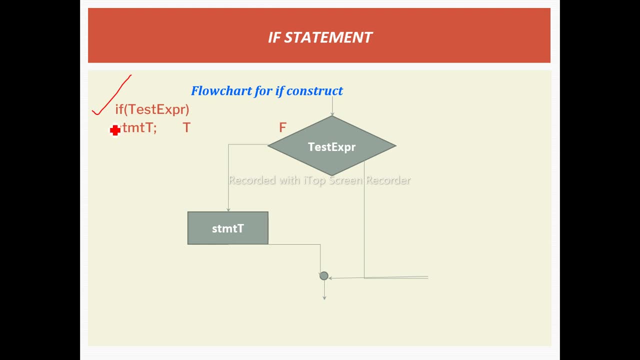 true, our block of statement or our if block statement will get executed, and if this condition become false, the cursor or control get passes to directly the next block. and here this is a diagram is given or flowchart is given for the if statement, in that, firstly, we need to give a test expression, that is nothing. 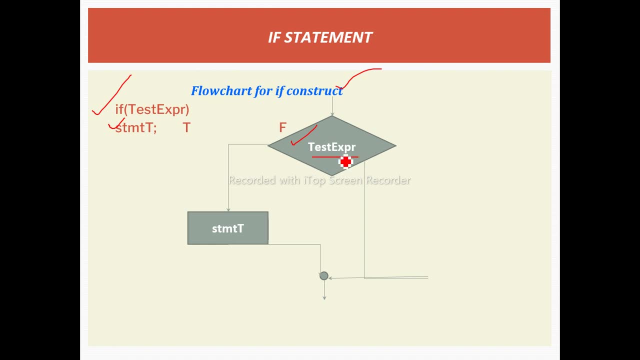 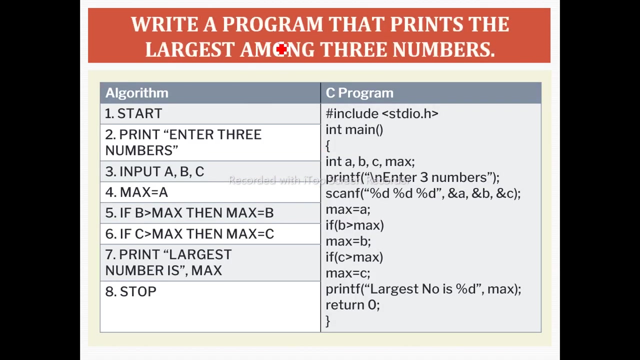 but the condition. if this condition becomes true, then and then only the block of statement will get executed. otherwise, if it is false, then the control get passed to the next state block. this is the program, by using if, condition or if control statements. here the algorithm is given firstly. 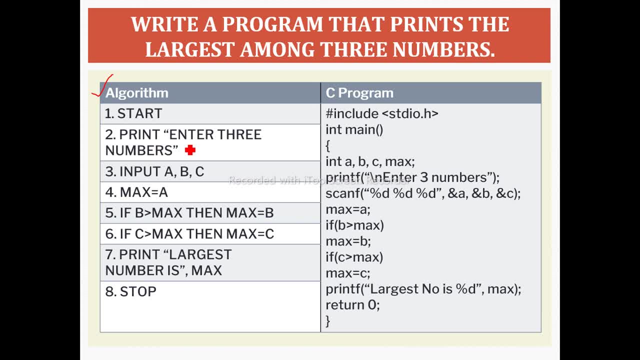 we need to start our algorithm. after that we are going to print the statement, enter the three number. so this program is used. or this program is for finding the largest number among the three number. so firstly, we need to display the statement, enter three numbers. after that we are going to take the variables value from the user, and that variables are a, b, c. 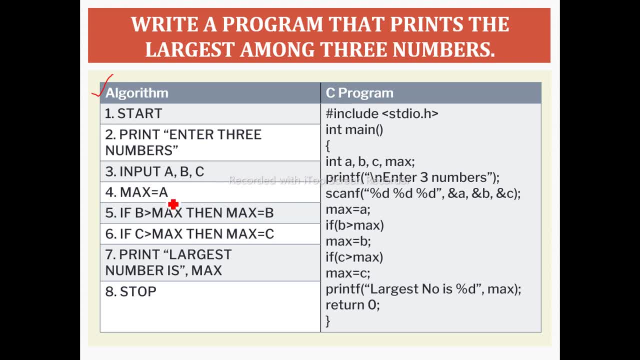 then we can, we are directly assigning the a value to the maximum variable or max variable, and after that, by using a if block, we are going to check the condition. if b greater than max, then we are going to pin or we are going to store the b's value into the max variable. if c is greater than max, 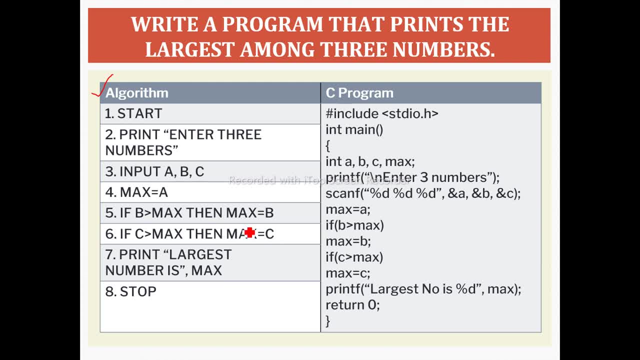 then we are saving the c value into the max variable and after end of this execution of this three statement, we will get the maximum value, that is the largest value among the three number, and we are going to display that by using the printer statement. so here the c program. 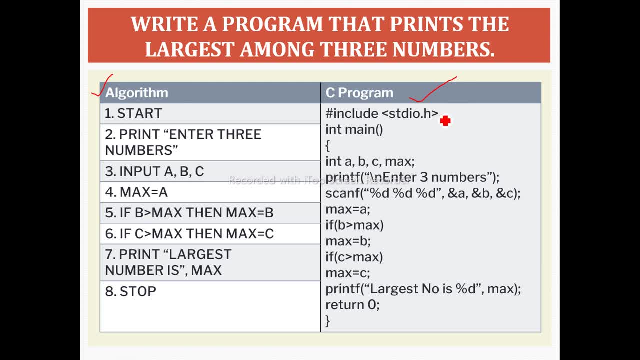 for the execution of this program. so firstly, we are going to enter the header file in a main program or in a main function. here this is the declaration of a, b, c variable to store the value of three numbers and to find a maximum value. we are going to take a variable max next by using 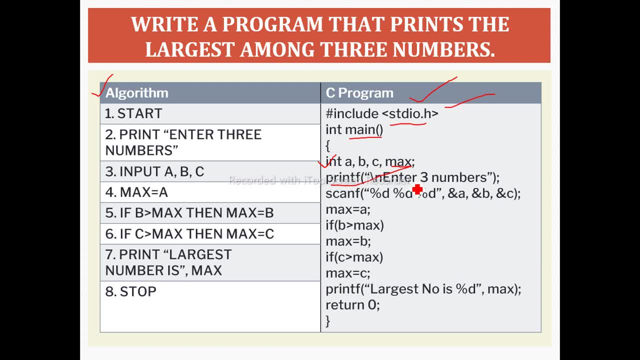 the pain statement. we are going to take a variable max. this is the declaration of a, b, c variable to. We are displaying this statement. enter the three number by using the scanf statement. We are going to save the value of ABC variable. Next, by default, we are going to consider A's value acts like a max value. 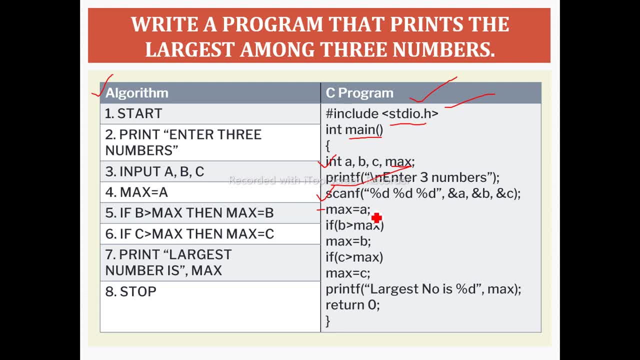 So to assign a value, max is equal to A. that is nothing, but a value will get assigned to the max variable. next, in if block, we are checking the condition, that is, whether B is greater than max. if it is true, then we are saving or assigning the value of B to the max variable. else again: 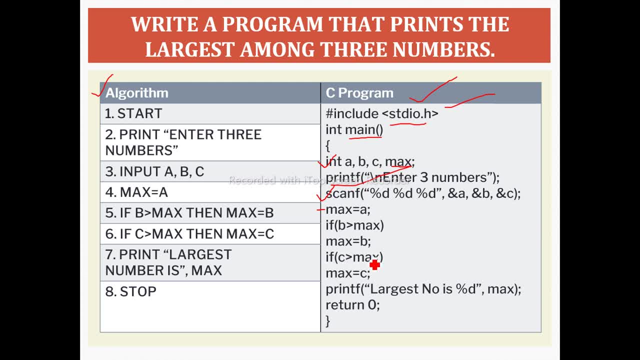 we are going to check whether that C's value is greater than max. if it is true, then we are assigning C's value to the max variable and by execution of this two statement, we will get the maximum value, whether it is A, B or C, and at the end we are going to display the 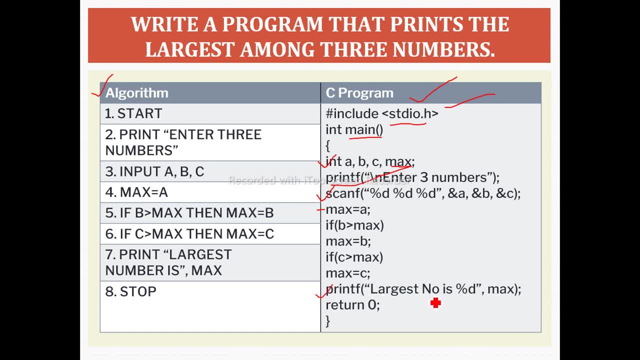 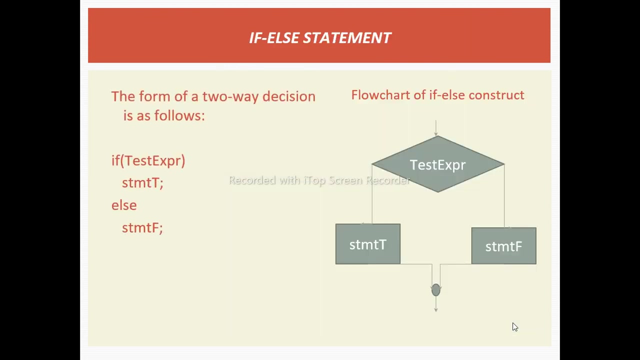 result by using printf statement: largest number is percent D. this is the format specifier, and by the using of format specifier we are going to display this max value. that is nothing but largest number among the three Next if else statements. so in this we are checking the condition and this if else statement, known as a two-way decision. 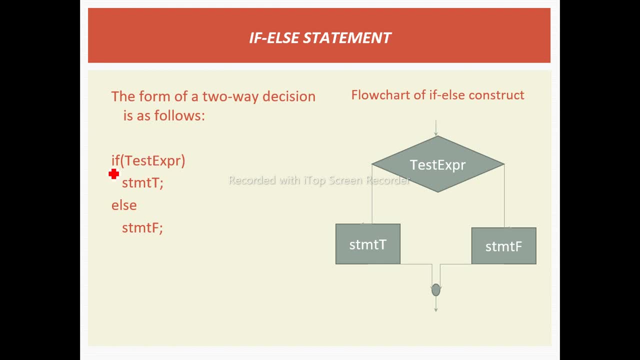 two-way decision is nothing. but if it is, if the condition becomes true, it will execute if blocks. if the condition become false, it will execute the else block. so that's why the statement is two-way decision statement. the syntax is given in a if condition. we are checking the condition. that is text. 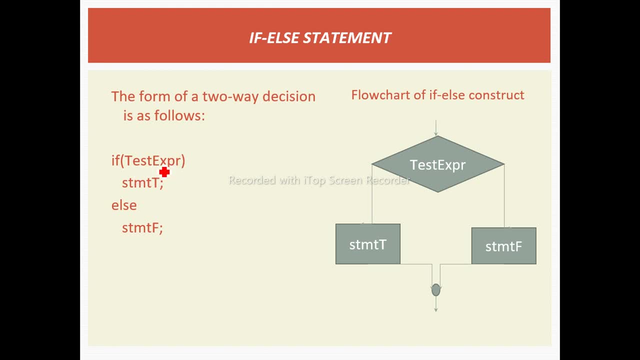 test expression. if this test expression condition becomes true, we are executing this if block. otherwise we are executing this algebra. the flowchart is given here: test expression. if this test expression becomes true, this statement tree T will executed. if this condition become false, it will execute the statement L. here the 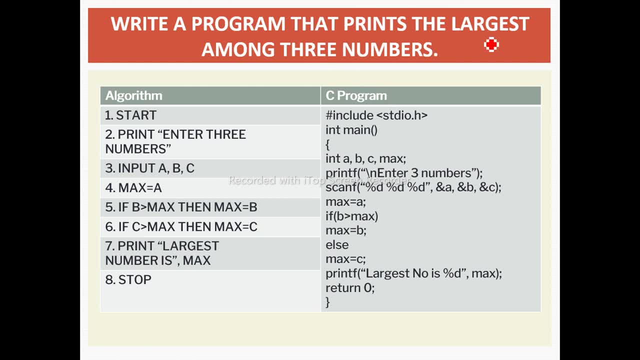 example is given again the same example for finding the largest number among the three. so a logorithmic them is same as the previous. the only change or difference in between here in a if statement. here, at both the places we are check, we were, we were checking if. 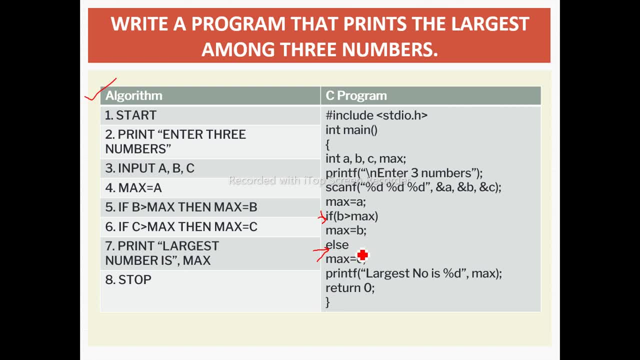 condition, but instead of the second, if here we place the else, okay. so that's why the if-else statement is two-way condition or two-way decision. that is nothing. but if our B is greater than max it will store the B's value into the Max variable, else it will replace them max value by C value. 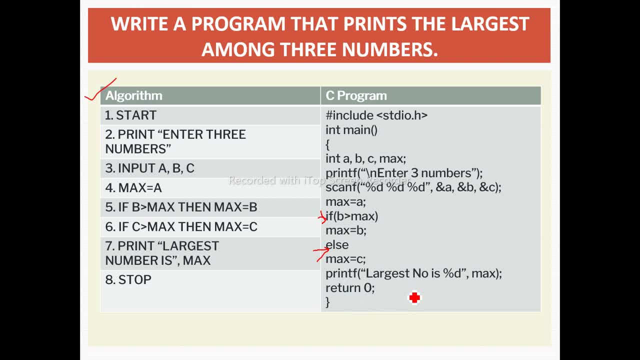 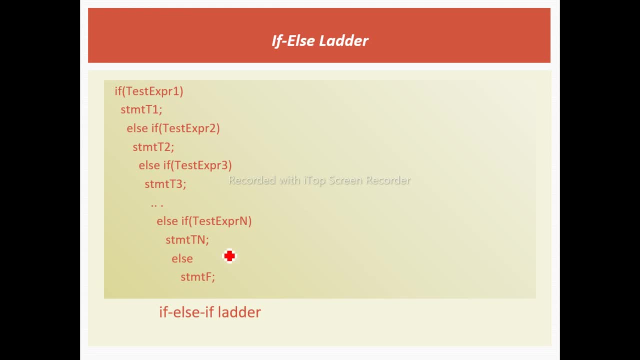 and by this we will get the largest number among the three. next is EFS ladder. EFS slider is nothing but with in a as again we are check, we are taking. if else block again that is nothing but after the else, again we are checking if condition again in that particular corresponding, else block again we are taking. 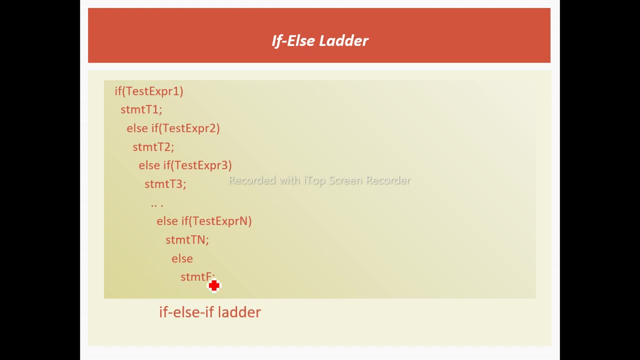 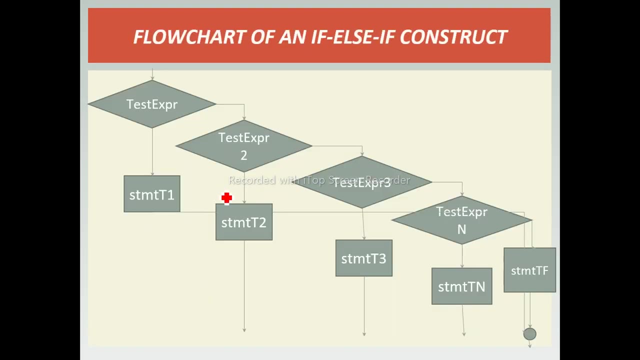 the if condition. so this is if else ladder, that is, if else condition within else block. so the flowchart is given for the if else ladder, or it also known as if else if. so that is first if condition. if it is become true, then we are executing statement t1. if it is, 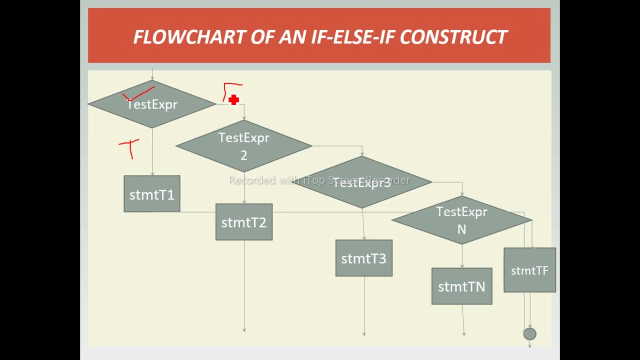 false, that is else block and within that else block. here again this if condition. but we are taking this: if block, within that if block, again the to condition: whether it is true, it will execute statement t2. if it is false, it will execute the next statement again. Who believe I guess we are taking if? 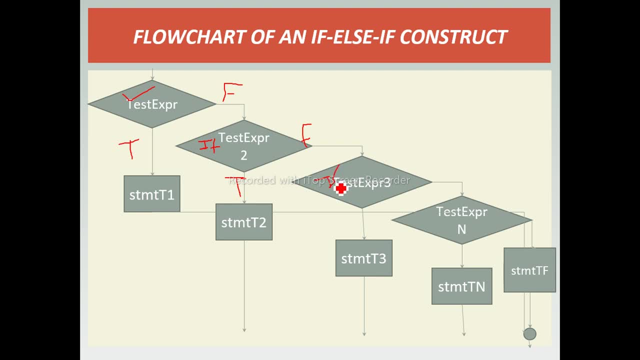 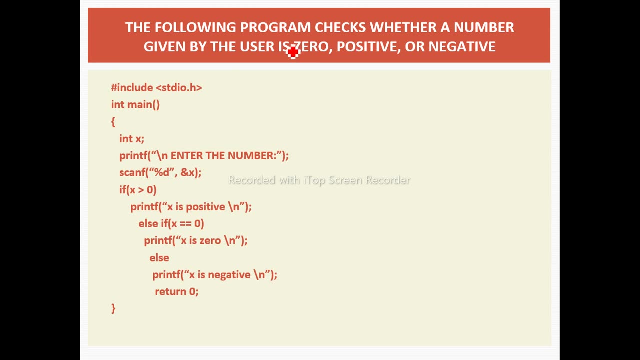 condition. so those plates for if else- my example is given. the program is to find or check whether a number given by user it's zero, positive or negative. that is nothing. but here we need to find out the three conditions. so firstly, first statement is header file. after that within a main: 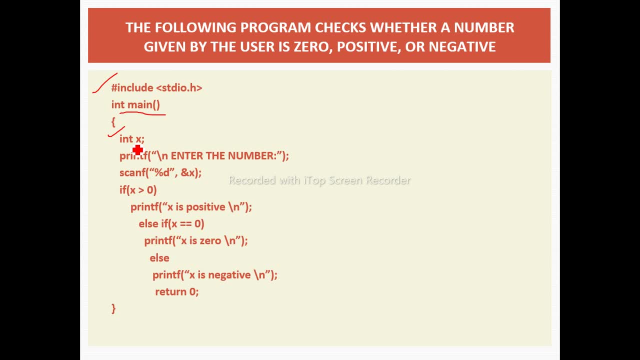 function. we are going to declare X variable or X number. after that, by user, we are going to take or store the value of X by using a scanning statement. so ampersand X. this will stores this user entered value into the X variable. after that we are checking whether that X is greater than 0 or not. if it is, X is if X. 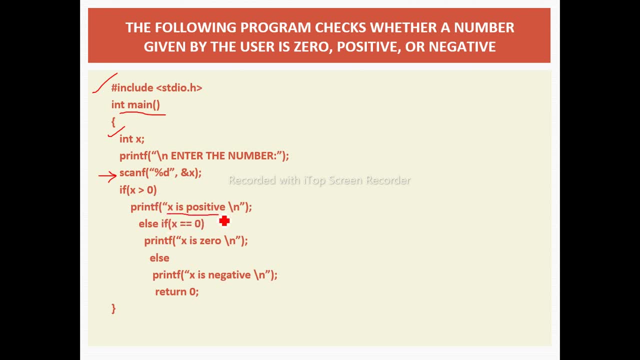 is greater than 0, we are printing X is positive, okay, again X, 0 say, but I need X, then it means it could be a 0 as well as its could be a negative. so in the S block again we are checking the if condition, whether it is 0 or not. if it is, X is equal to equal to 0, equal to equal to. 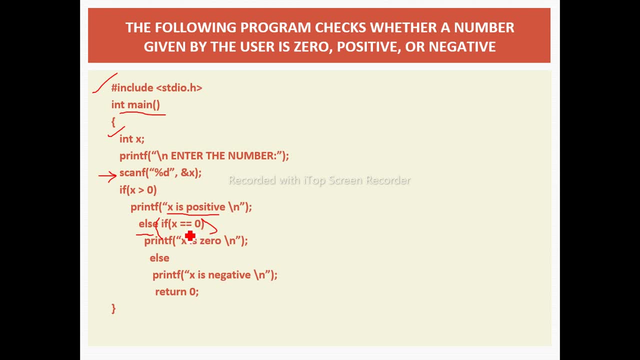 sign is used for the comparison. so if our X is equal to equal to 0, that is nothing but X having the value 0, then we are printing X is 0, else we are printing X is negative. after that we are returning the zero value to the main statement. and here we completed. 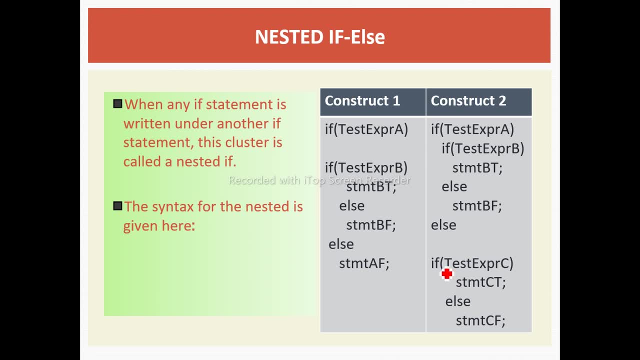 our program next is nested if else. so nested if else is nothing but within a if block. again we are taking if else condition. so when any if statement is written under the another if statement, this cluster is called as nested if, but we are also calling it as a nested. 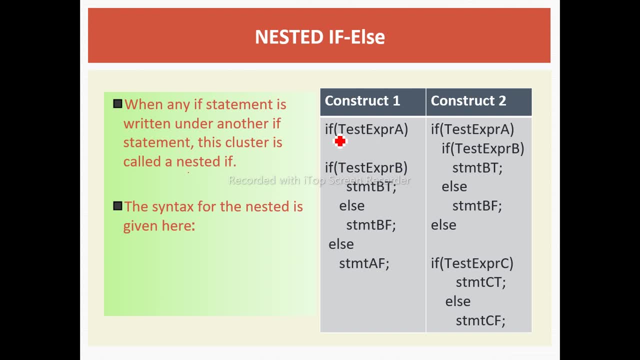 if else. so the syntax is given. so this could execute it in two way, that is, only by using if statement and as well as by using a else statement, and in both the if and else statement we are using if else block. ok, so here in 1 we are using only the if statement and within that if statement we are using if else block and 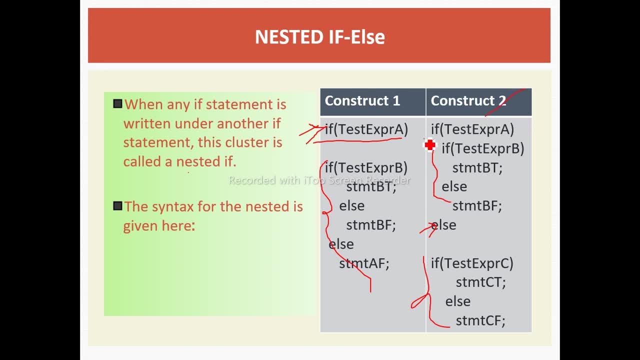 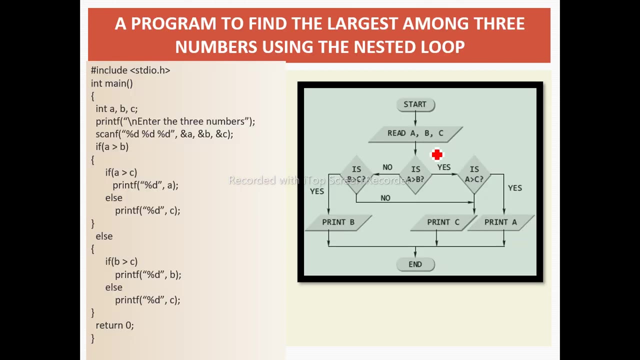 in construct 2, within the if block we are taking if else statement, or if else block, and again in else statement or else block we are taking if else. next is: this is the example is given for nested if else. so the program is to find the largest number among the three by using the nested. 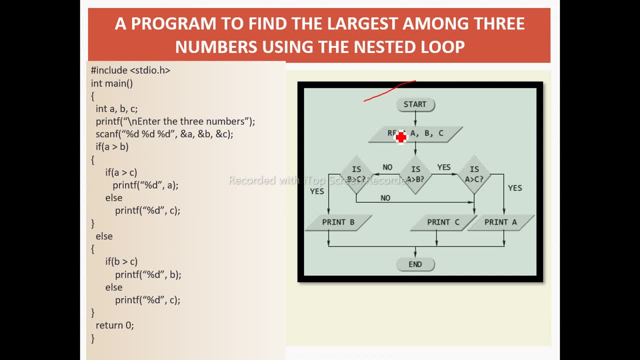 loop. the flowchart is given. firstly we are going to read the three value ABC. after that, here we are checking: is a is greater than B? if a is greater than B, we are checking. if a is greater than B, we are checking. if our this condition becomes true, we are checking whether a is also greater than C. other a, B. 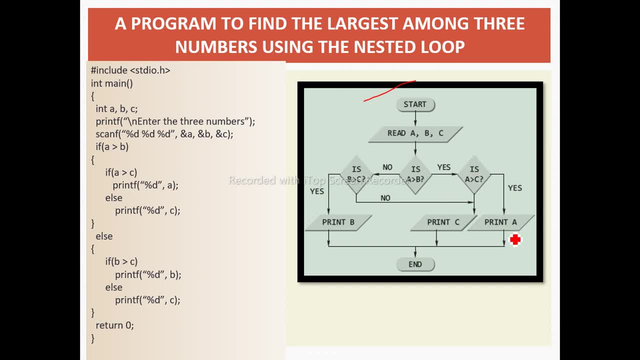 say be greater, hence he say: be greater a, then it means we are printing: a is greater. okay, if a other B say, but I had but, but C said Chota, hey it means C is greater. and other Mira egg B say, but I mean again, we are checking: B is greater than C over B. Mira C say: be murderer the Audi. a say B, but don't. 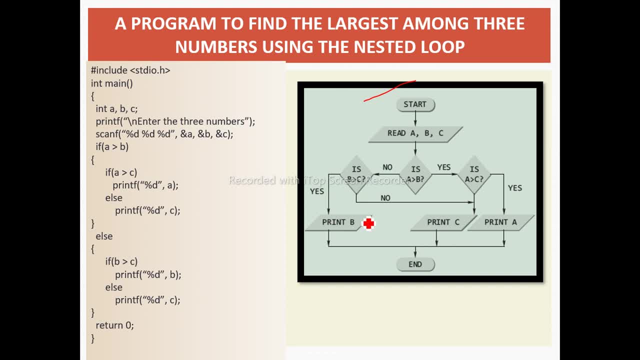 than definitely be the largest value. so we are going to be included. so to execute this block we are taking nested if else. so here in if block we use if else, and again in s block, again in s book we are taking he says so this becomes a formal figure. so the last to using if is also a bound. 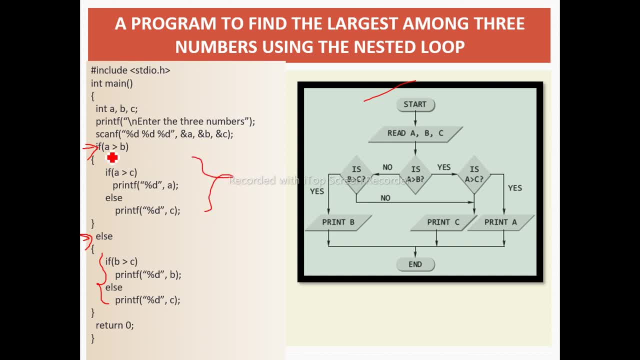 our nested affair. so firstly we have to check A is greater than B if A is bigger than B. so at the same time we are checking A is bigger than C or not. if it is true, then we are printing: A is greater. if A is bigger than B but not bigger than C, then surely our C is largest. 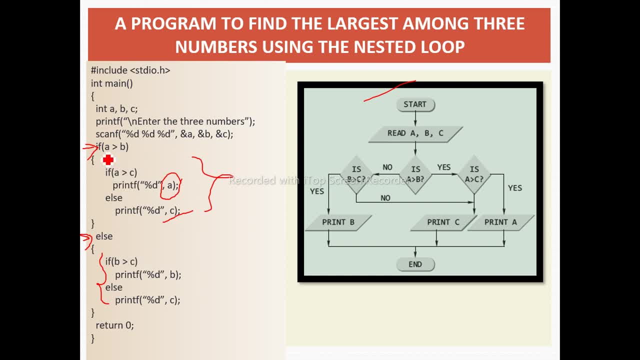 number else. if our A is not bigger than B, it means B is greater than A. if B is greater than A, we are checking: B is greater than C, yes, then B is the largest number, else C is the largest number. and at the end we are printing or returning the value of main function. that. 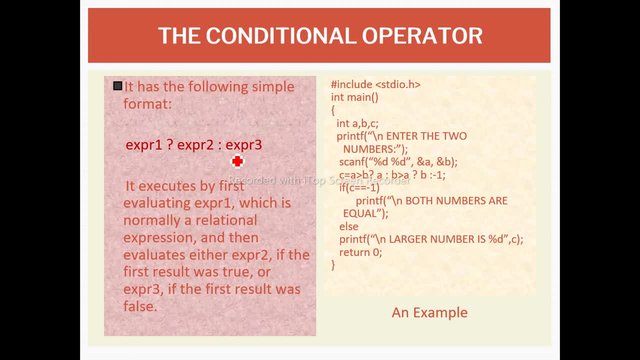 is 0. next is conditional operator. so condition and condition operator is nothing. but here in this conditional operator we can give one condition. if it is true, then expression 2 will get executed. if this condition is false, expression 3 will get executed. so the description is given. you can execute by the first evaluating. 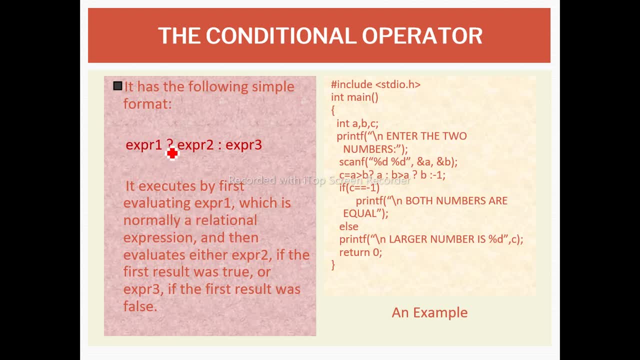 expression. so expression 1 is our evaluating expression. okay is, the value of first expression is true. now here we arechthing one is true turned to being. because expression one worked, then expression 2 will get executed. if its value is false, then expression 3 will get executed. 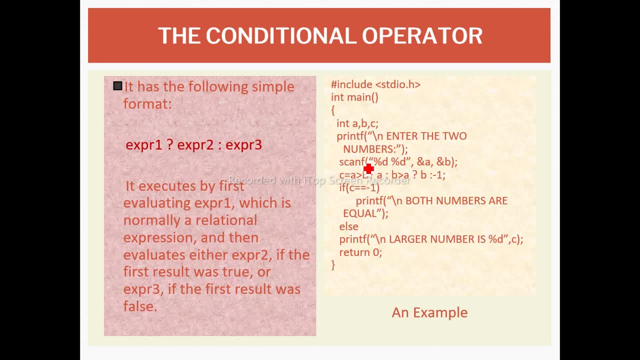 so here the example or program is given. firstly, we are going to define the header file within a main block. we are going to declare the three variables: ABC variable. after that by using the printf statement, we are displaying the message. enter the two number after that here by using: 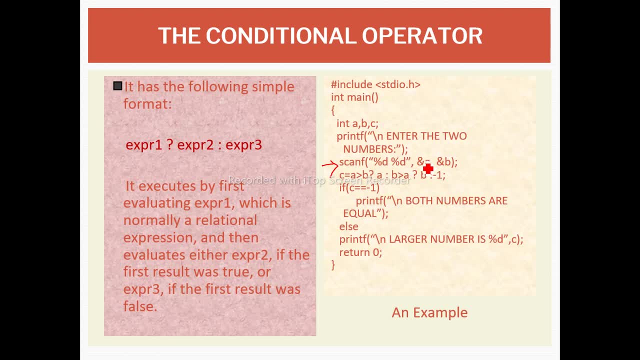 the scan if we are taking the value of a and B from the user. so ampersand a, ampersand B, it will scan the value and it will store the value into the a and B variable. again. now this is our conditional operator, so here we are checking if 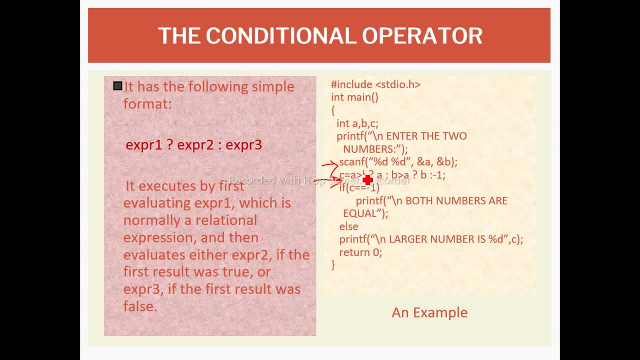 whether that a is greater than b. if a is greater than b, then we are storing that a's value into the c variable. if it is greater, then we are again checking whether that b is greater than a, if it is true. if it is true, it will. 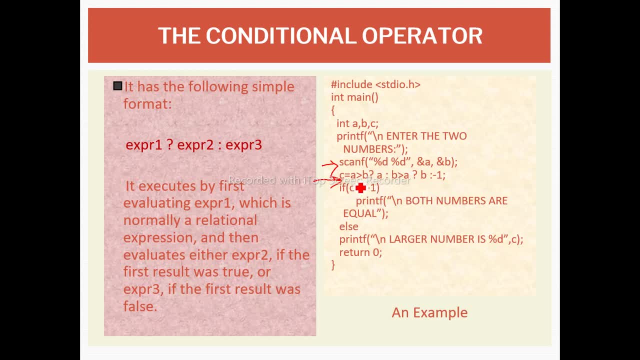 execute this statement. see here: firstly, we are checking a is greater than b. yes, then a execute. if a is not greater than b, it will execute this statement again. in this statement it will check whether b is greater than a. yes, then it will print b. if it is not, it will print minus 1. so if c is, 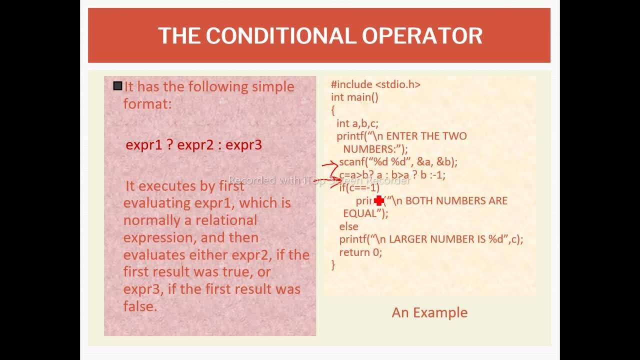 equal to equal to minus 1, that is, it will compare the value of a and b. so if c is equal to equal to minus 1, that is, it will compare the value of c. if c having the minus 1 value, it will display both the numbers are equal. else it will display the message larger number is c. so this is here we. 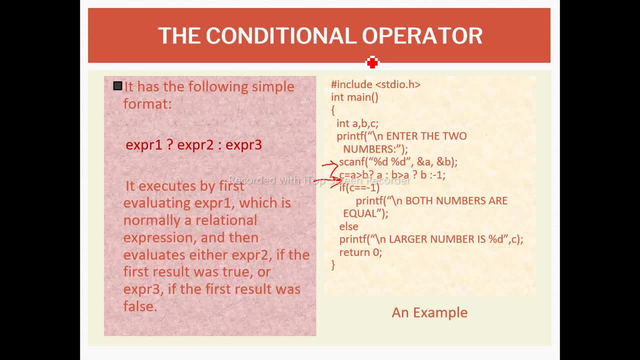 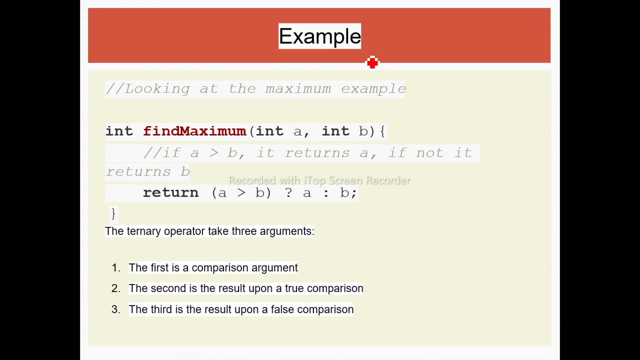 completed conditional operate conditional statements. in that conditional statement we have learned three, that is four statements. that is if block, then if else block, if block is one-way decision. second is: if else block, that is two-way decision. next is: if else ladder and nested equals, these are the multi-way decisions. so here again the same example is given for the conditional. 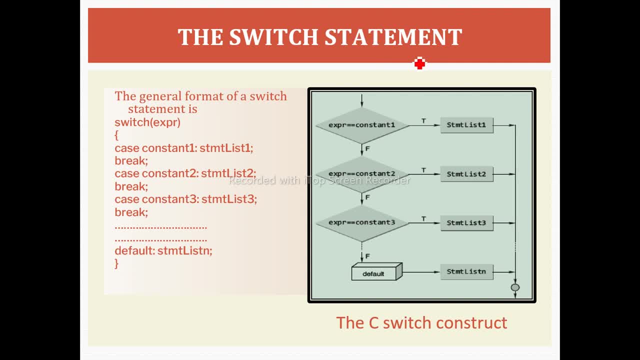 operator. next is switch statement. again, switch statement is by using a condition. so the syntax is used in a TV switch statement. here we are giving the expression or condition and for the corresponding condition we can give the multiple cases or multiple block of statements. that is case 1, Case 2. 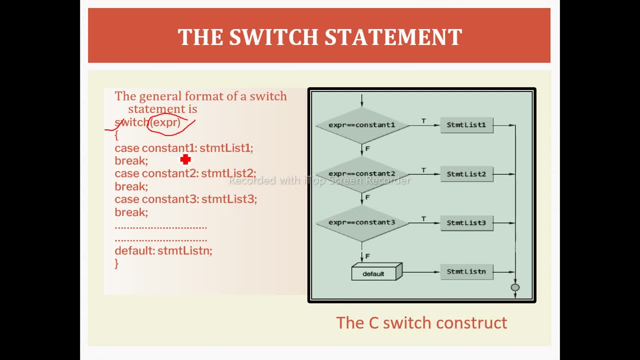 okay, three like this. and every time, with the cases, we can execute this block of statements. and every time, whenever we compete, the 1 block of statements is gebe down this. then there can be an intuitive way of getting the, the economic contribution over the statements to beだから. except with this, we will do the following: with the civilization working so, 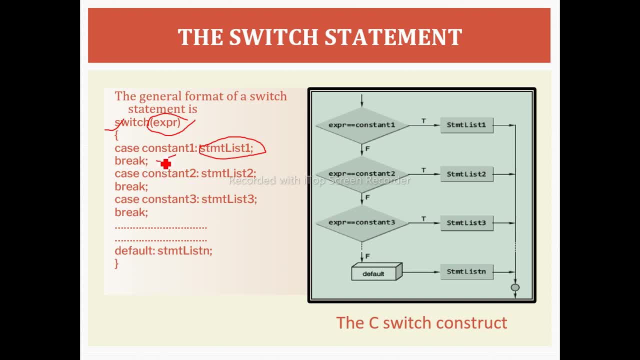 every time, whenever we complete the 1 block, the 1st time. okay, if were participating, we must participate. a detail you must say on a conflict. finally, touch this sentenceえて. static to this sentence. as a this restaurant yina read the block. we need to give the break. so break statement will enter up the whole. 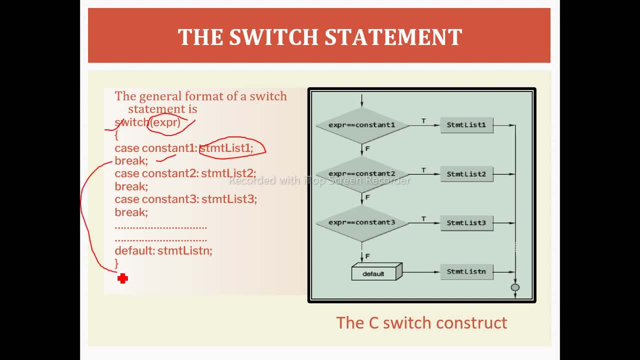 condition and the control will get come out of the loop. so here the same flow chart is given on this case 1. in case 1 we are going to give the condition. if it is true, then it will execute the statement back again. if it is false, it. 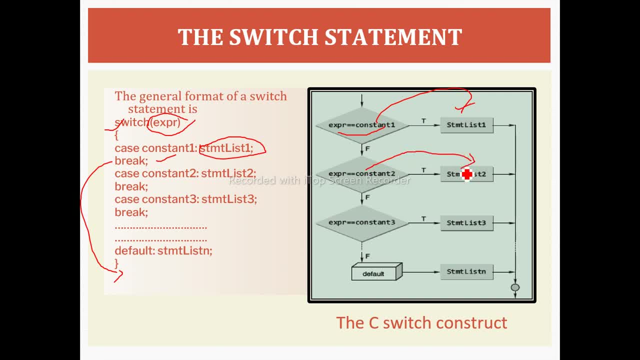 will check for this case 2. if case 2 will get match, it will execute the block of statement and in this switch case or switch statement, we need to give the default statements, which is compulsory. okay, isse kya hoga agar humara koi bhi conditions match nahi hota hai with the? 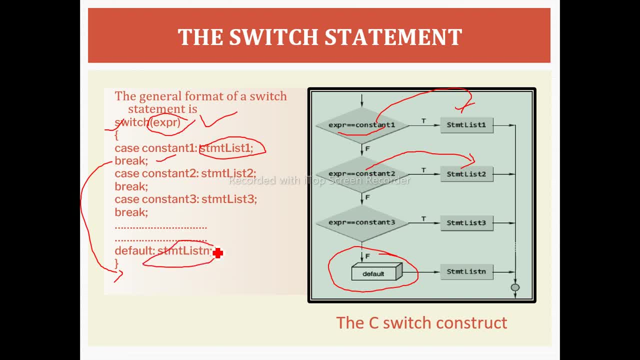 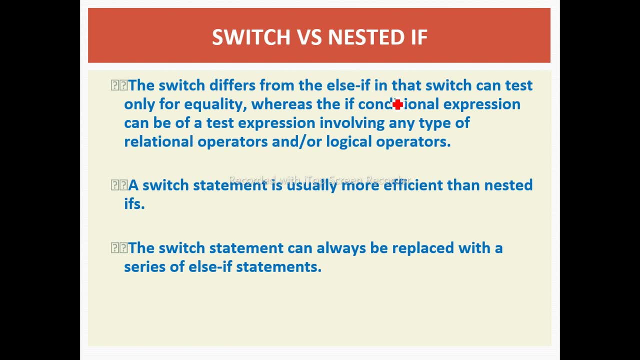 cases it will execute or the control will get passed to the default statement and it will execute the default block of statement. so the switch differs from the if-else in that switch can test only for equality, whereas if-else condition can be test expression by using the true and false. 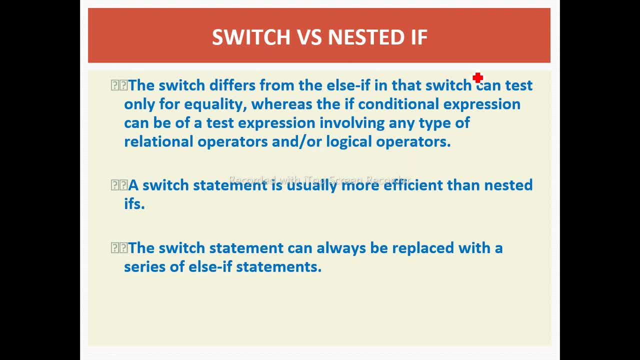 so switch se kya hoga? equality check hogi, but if-else se kya hota hai, the expression will get check whether it is true or false. next, a sweet statement is usually more efficient than the nested equals. why? because in a switch case or in a sweet statement, we can give multiple cases at. 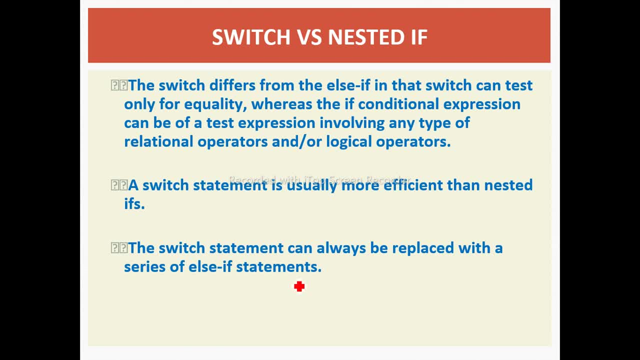 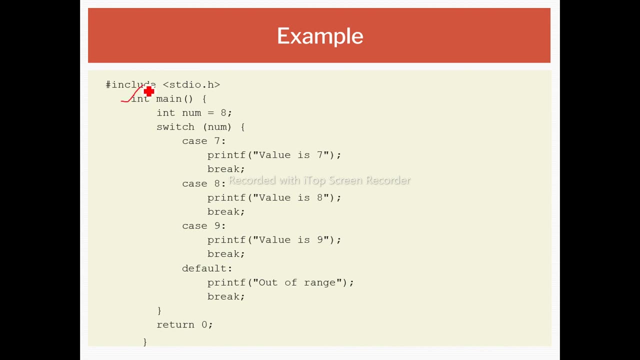 the same time. so see switch. a statement can always be placed with the series of else block. so the example is given here. we are going to start the program and we are initializing the num variable by 8. okay, and we are passing this num variable to the switch block. okay, so now. 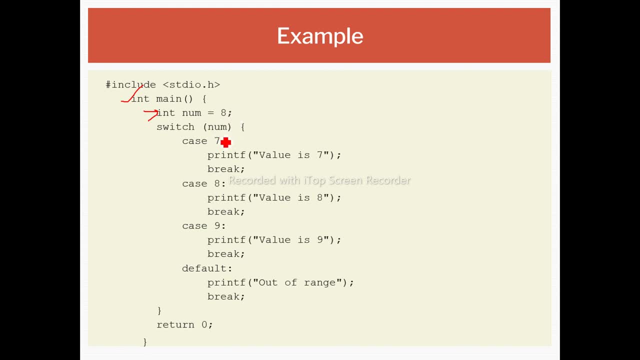 currently num having a value 8 and it will match with the case 8. so a only case 8 will get executed. that is, it will print the value is 8 and the break statement will execute it. that is nothing but control comes out of the loop of switch block and it will return to the main. so this program ka output. 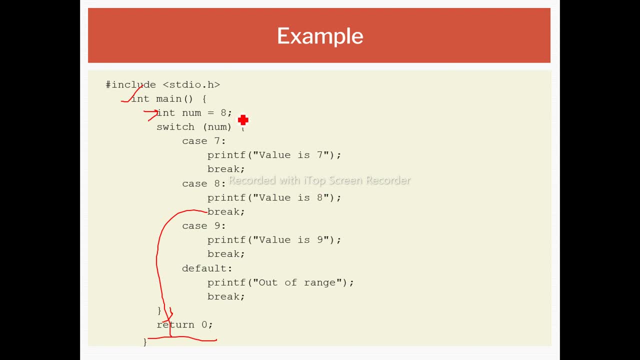 kya hai. value is 8. okay, now consider if i replace this num variable value to the 9, 9, so it will execute only the case 9. why? because value is 9 will get printed and break statement will get executed, agar num variable main main one store. kya hota? so case 1 aise kahi bhi nahi hai. so that is nothing but. 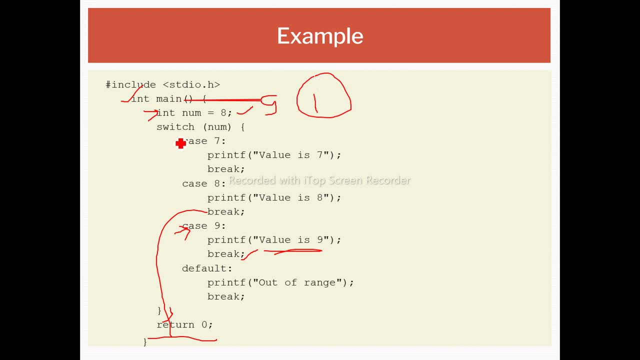 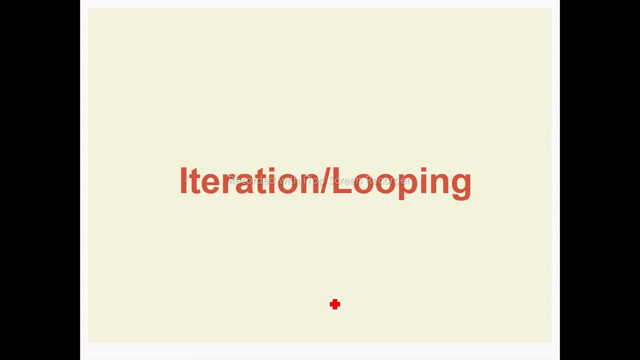 this case of value 1 will not get matched with the any of the cases. so jo bhi default statement hai, that default block of statement will execute it. so again, many num is equal to 1. store kya what will be the output out of range? so here we can t completed conditional operator or conditional. 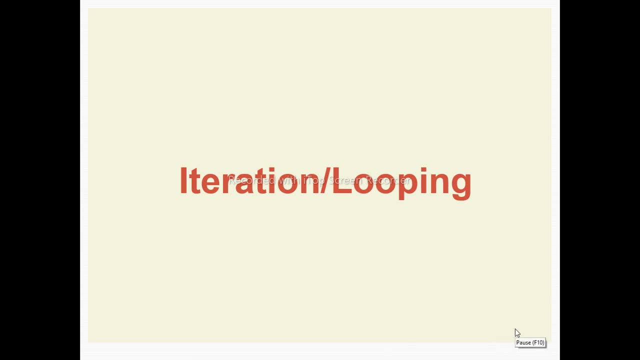 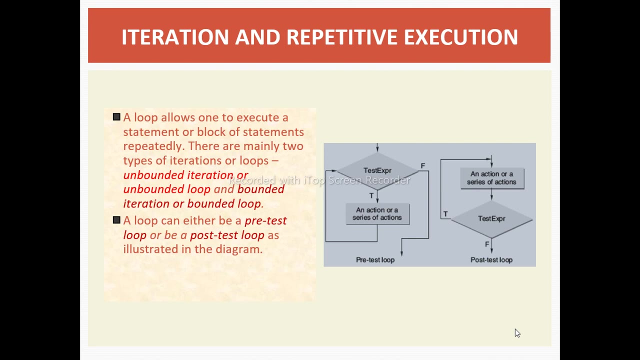 control statements. so next block of statement or control statements are iteration statement or looping statement. in this the block of statement or a block of code will get executed in repetitive manner. a loop allows one to execute a statement or a block of statement repeatedly, that is, in an iteration manner. there are mainly two types. 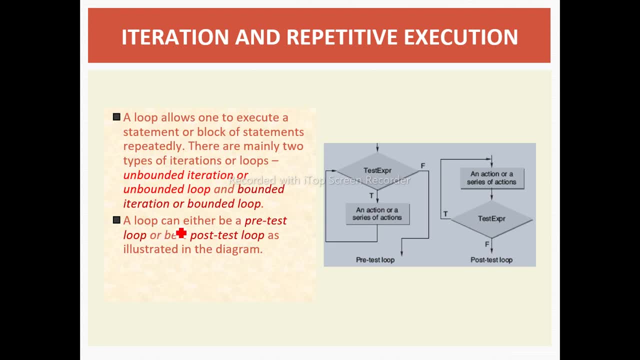 of iteration that is unbounded and bounded. a loop can be either be a pre-test loop or posted loop. pre-test means first check the expression. if it is true, then and then only block of statement will get executed, and post test means compulsorily it will execute in. 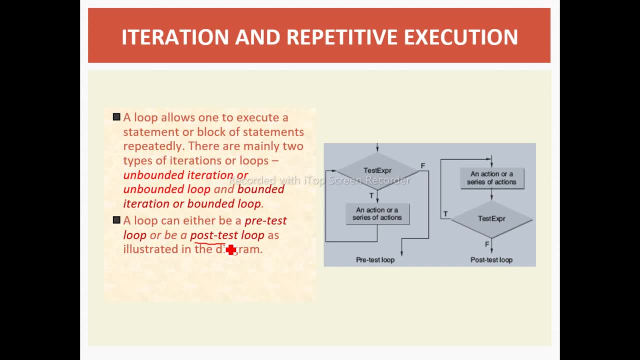 at once and after that it will check the condition. so the diagram or flowchart is given for the pre-test loop and posted. so what will happen in pre-test? compulsorily at the first time it will check the expression. if it is true, then, and then only, it will execute the block. 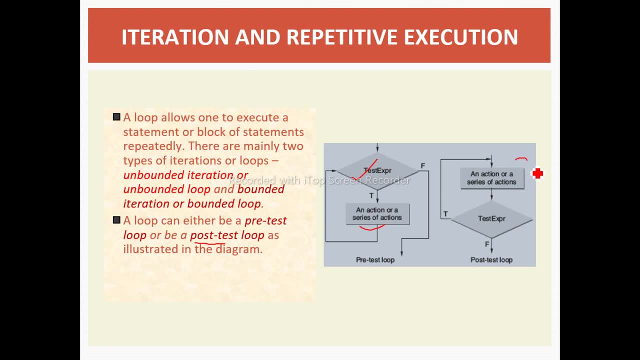 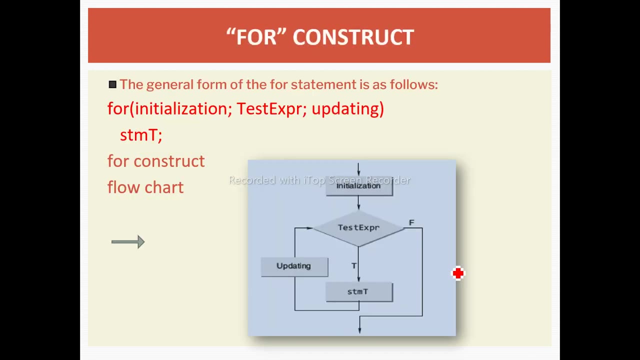 of statement. so what will happen in post test? the block of statement compulsorily executed at once, and then it will check the condition. so now we will see this looping or iteration one by one. so first is for construct or for loop. the general form or syntax is given for loop. so in a for loop, firstly we need to initialise. 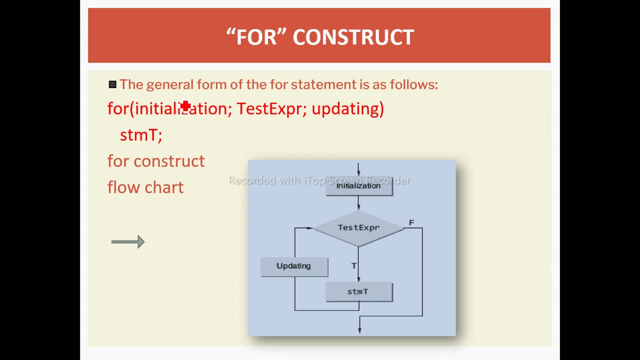 the variable that for that particular variable here we are checking the test or expression and we are updating the value of that initialize variable. so in a updation we can increment the value of variable and or we can decrement the value. so the flow chart is given initialization of variable. for that variable checking a. 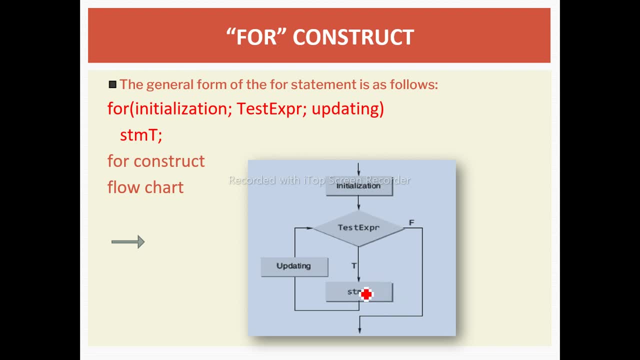 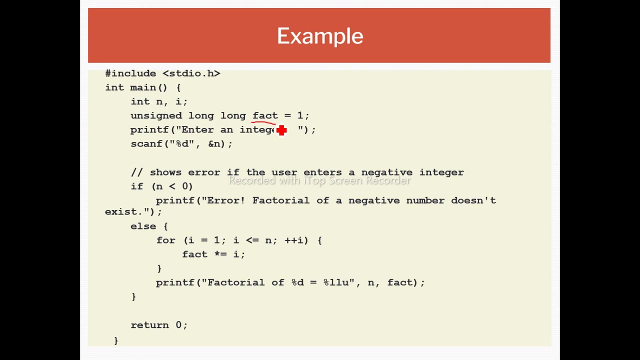 condition. if it is true, execute the block of statement. if it is false, we will come out of the loop. okay, and after checking the condition, we are updating the variable in updation. we can increment it or we can decrement it. now we will see the example. so we have taken the fact variable having the value 1 by 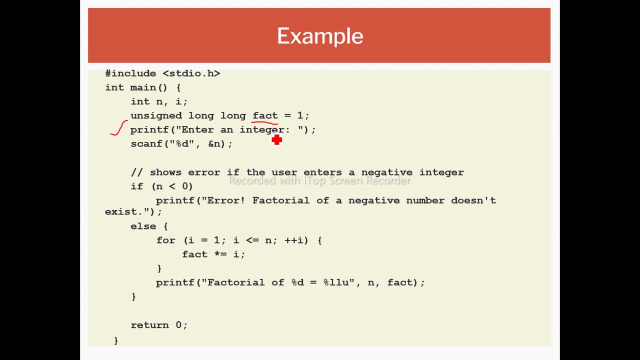 using a printf statement, enter an integer. here we are checking or finding the factorial of a number. so to find as factorial, take the value from a user by using a scanf statement. okay, so firstly we will check that whether that number is less than 0. why? because whatever is negative number and 0, we are not finding its factorial. 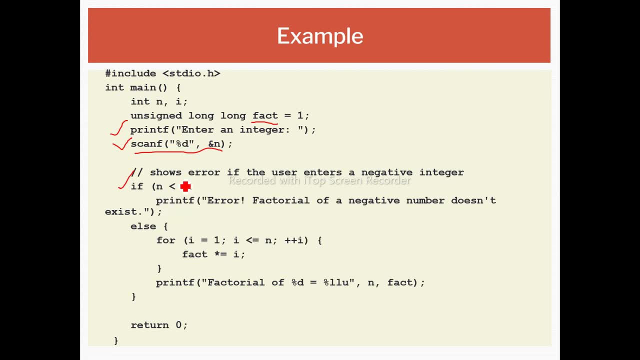 out. okay, so to find a factorial of a number, we need to firstly check whether that number is positive or not. if that number is positive, then and then only we can find out the factorials. okay, so if it is positive number, the control comes into the else block and here we will start the execution of for loop. so in a for loop, 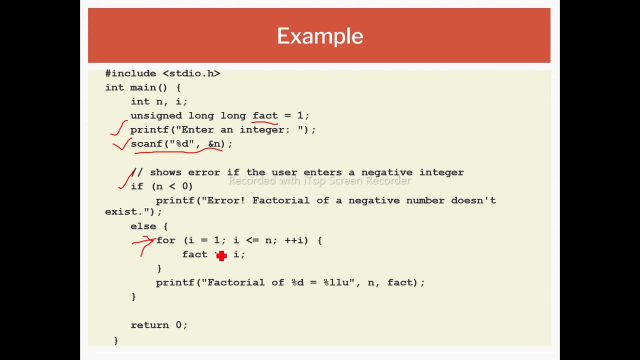 here we have initialized it. this is the initialization of for loop and we have developed a variable of for loop, revolution, and for this i is equal to 1. that is initialization part and we are declared this I variable here. okay, next, for this particular variable only. we are checking. so in this program half also. 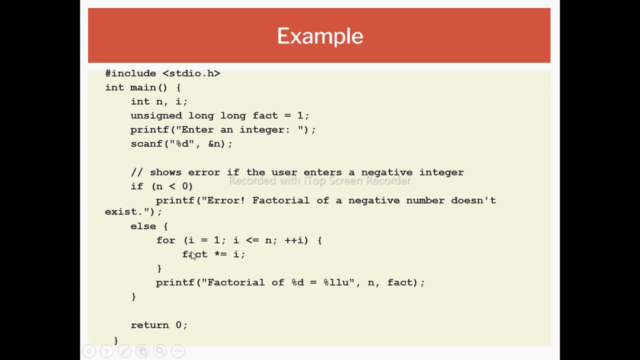 in Fallout we are fishing by using a forward loop, so in a for loop. firstly, we are initialising by using the for loop. we are initialising a value of for loop. so in initializing the i variable and for that corresponding i variable, checking the value, whether that value is less than is equal to n. if it is true, then we are performing the block of. 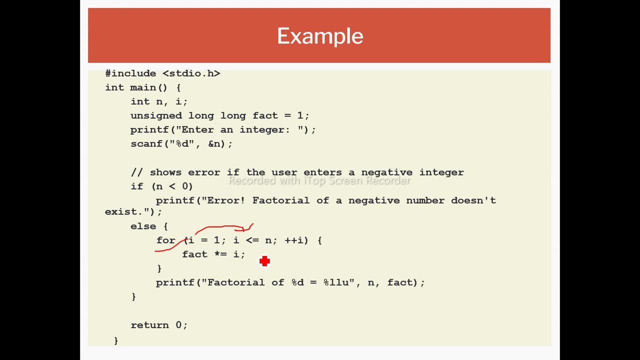 statement that is fact into equal to i. it means that it means that fact is equal to fact into i. so that's why that into equal to sign will be combined here. so if this i condition becomes true, that is, i is less than is equal to n, we are performing this and again we are incrementing. 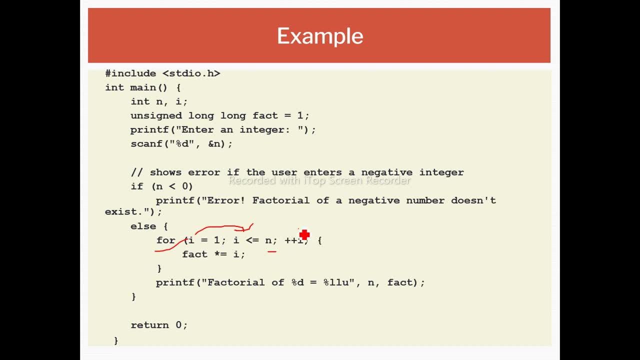 that i value. okay, why? because here the updation is required. and until this condition become false, okay, if it is um, um, if this condition become false, it will come out of this for loop. that's why this for loop, known as a loop or iteration block, and at the end of the statement of for loop or at the end of the for. 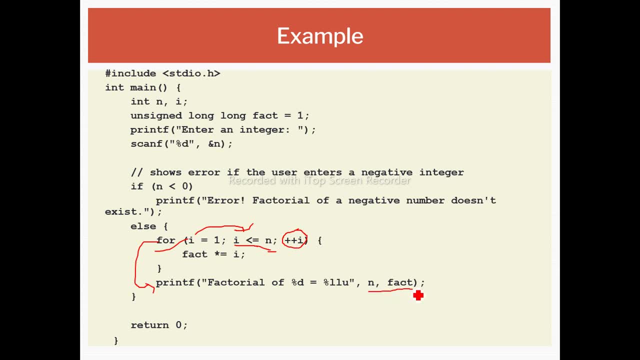 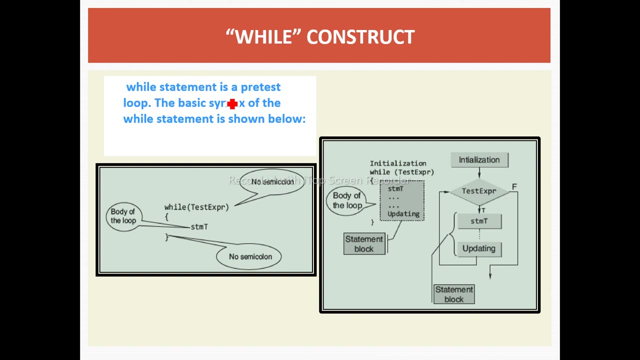 block of for. it will display the result that is: factorial of n is equal to llu, llu. this is the format specifier for unsigned long, long file. is that clear? so here we completed the example of for loop. next is while loop. so in a while loop, while statement is pre-test loop. 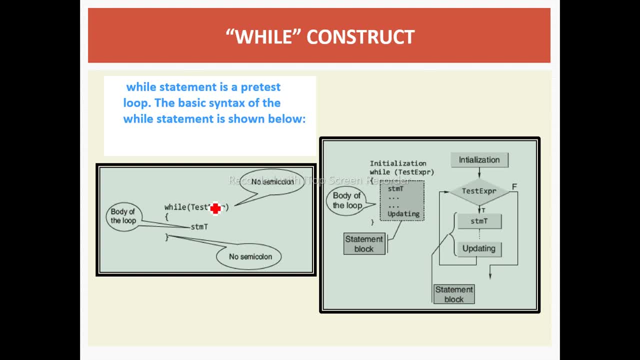 pre-test is nothing, but firstly we are checking the condition and after checking the condition we are executing that block of statement. so the basic syntax of while statement is shown below as like the same if statement. here we are checking the while condition, but but the only difference in 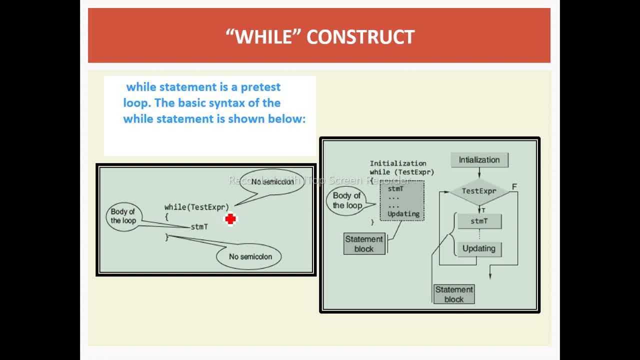 if and the while is that until the condition becomes false, we are executing this while loop and if make a if is the only one way execution or one way implementation, and while is nothing. but here we are checking the condition multiple times until that condition become false, and while is the pre-test flow. why? because previously we are 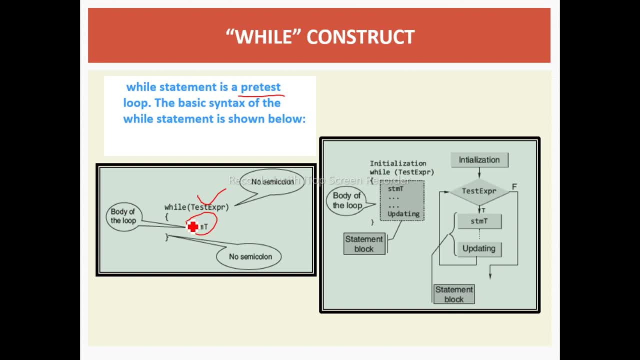 checking the condition and after that we are executing this block of statement. so the flow chart is given: firstly, we are initializing the value of variable. after that we are checking the condition. if this condition becomes true, executing block of statement. after that we are updating that variable value. 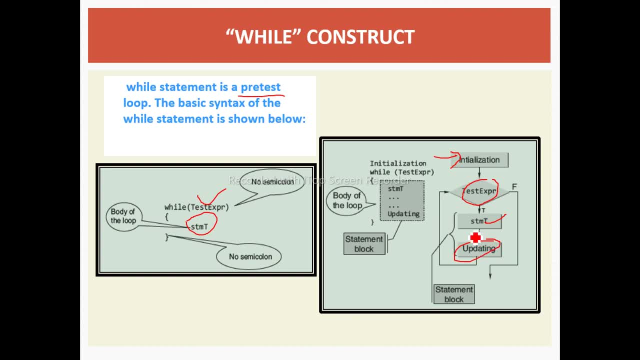 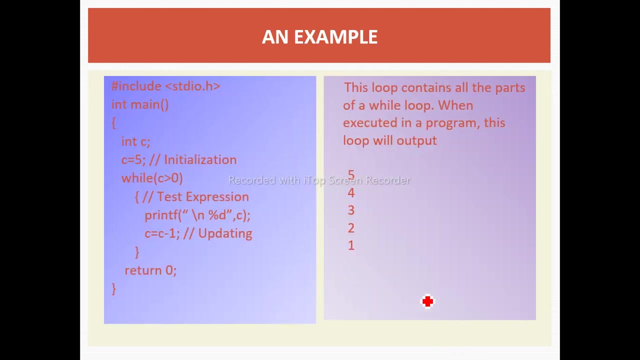 that is, if we can increment as well as we can decrement the value. after that, again, we are checking the condition up till the condition become false. whenever this condition become false, the control comes out of the while loop and next block of statement will get executed. so now we will see the example or the program for the while loop. so here, 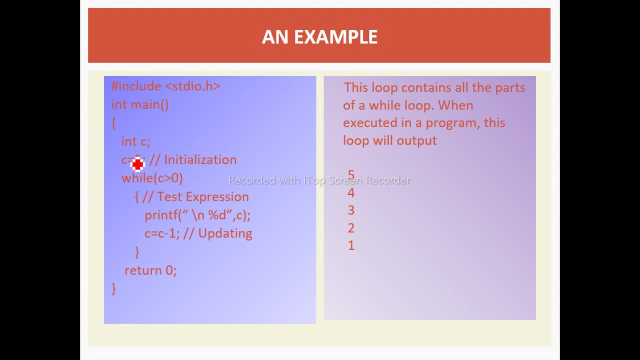 we are displaying the number from variable to the one or in a decrementing manner, so in the main block or main function. firstly, we have in declared the c variable. after that we have initialized it value to the 5. okay, and if we wanted to display the 5, 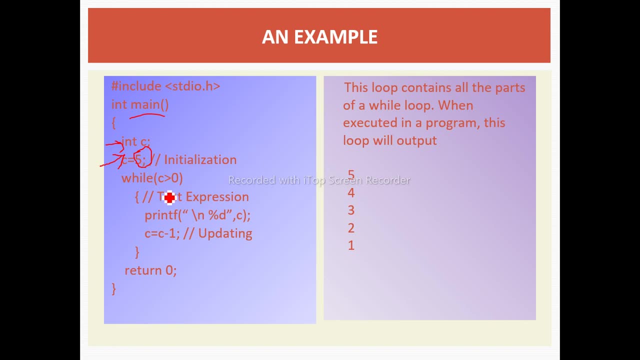 display the number in a decrement manner. here we are checking the condition. c is greater than 0, matlab jab tak c hamara 0 nahi hota tab tak. we need to perform this operation or we need to execute this block of statement. okay, so inside the while loop. firstly, we have taken the c value. 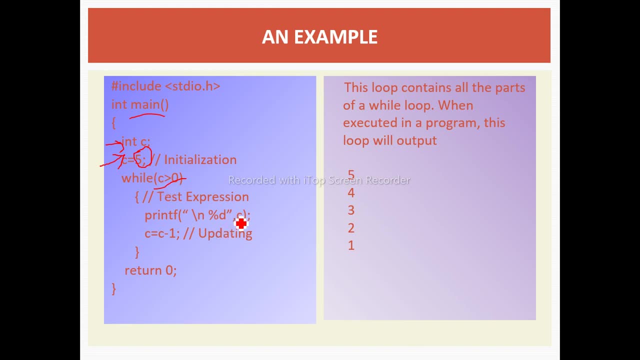 as 5. so 5 is greater than 0. yes, it will print the c value. that is 5. okay. next, here, at the next statement, we are updating the value of c. that is c minus 1. it means we are decrementing that c value by 1. again, it will check. 4 is less than 0. yes, it will display the 4 value. 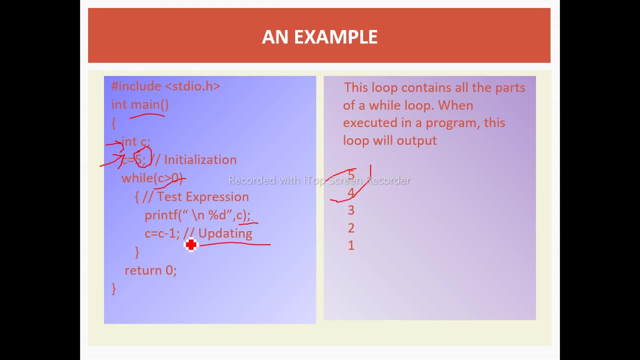 4 is less than 0: yes, it will display the 4 value. 4 is less than 0: yes, it will display the 4 value. next again, the value c value will get decrement by 1, so 4 minus 1 it will become 3 again. 3 is. 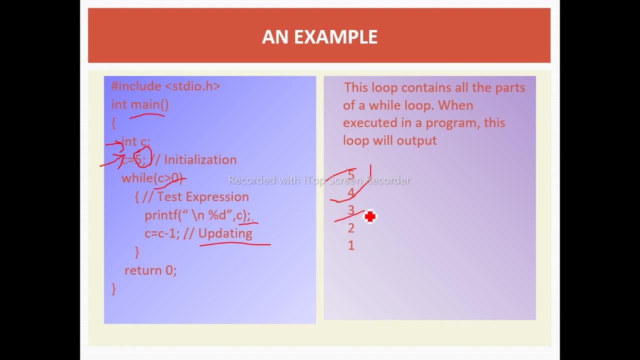 greater than 0. yes, we are displaying that d value again. we are decrementing that c value by 1. 3 minus 1 it will become 2 here. here we are checking: 2 is greater than 0. yes, we are displaying the 2 again. we are decrementing that c value by 1. 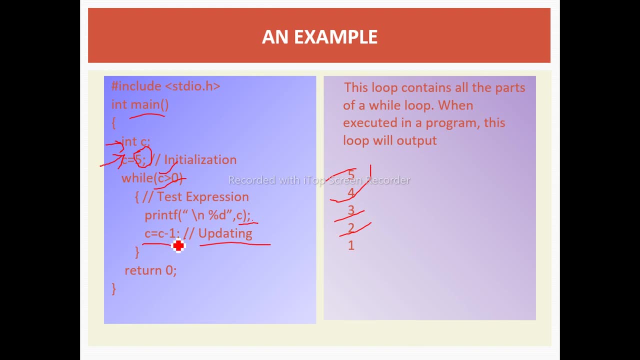 that is 2 minus 1, it will become 1. 1 is greater than 0. yes, we are displaying the c value, that is 1, and again we are. we will decrement that value. that is 1 minus 1. it will become 0. again here we. 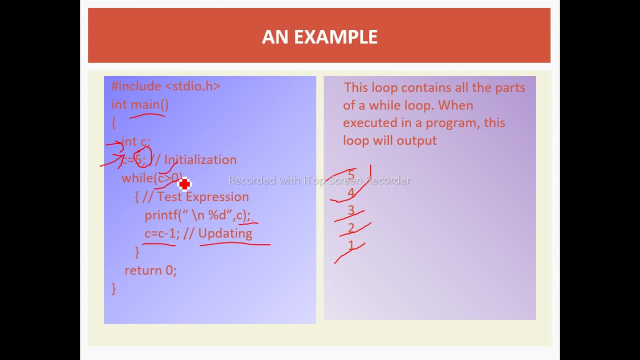 are checking the value whether c is greater than 0. no, it becomes false. so we will come out of the loop and add next block. next statement is return 0. so return 0 will return the 0 value to the main function. and here we completed our program. okay, so the while loop is nothing, but we are checking. 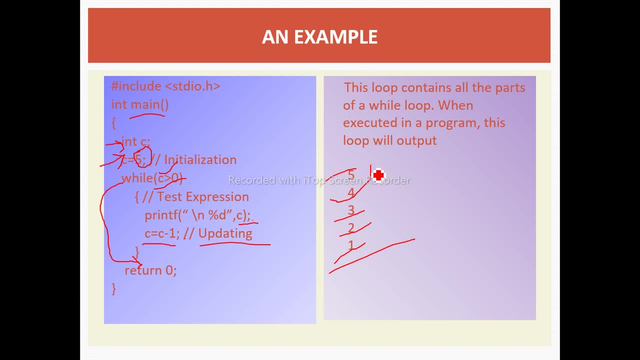 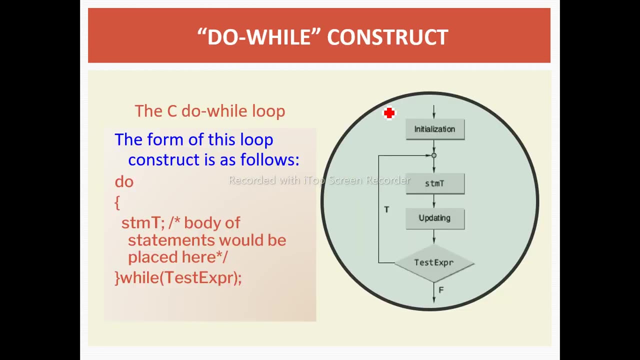 that condition unless and until that condition become false. if that condition is true, we are executing that while block of statement. next is do while, do while is our post test expression. post test expression is nothing but once. we will execute the condition. after that we will check the condition. so in a while, do while loop, the block of statement will get executed once, any, any which way. 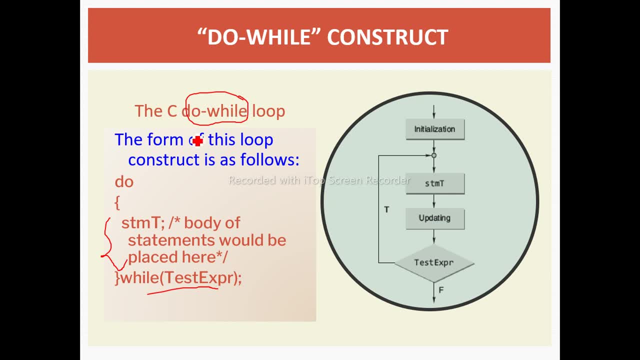 whether that condition is true or false. any which way, the condition or block of statement will get executed once. so that's why this control statement, known as a post test expression. so here, same as the previous. firstly, we will initialize the block of statement. so let's firstly learn this syntax. so 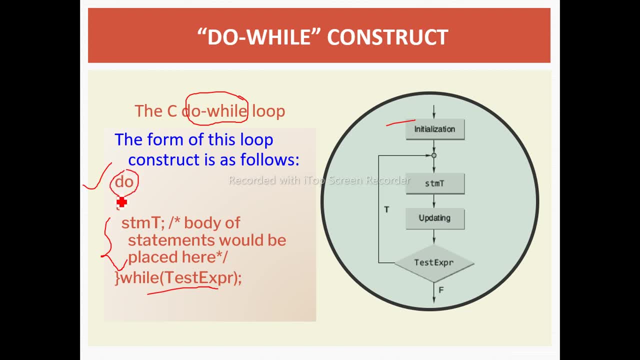 syntax is: first give the do keyword, after that in a do block we will write the block of statement, and after the end of the do block we will write the while expression. and in this while expression, here we will give the test expression. if it is true, our do while block will get executed. 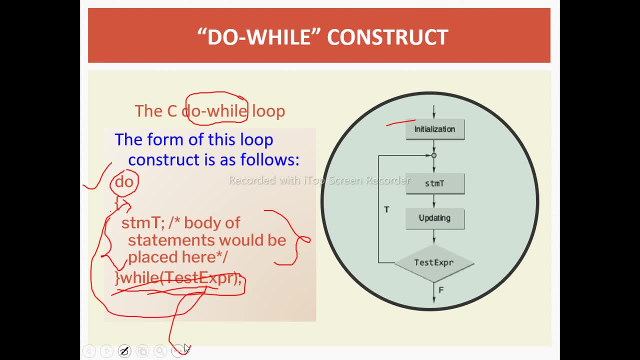 if it is false, the loop come out of the block. so here, first, initialization of variable. again here, this is our do do ka matlab kya hai? the test or statement will get executed once in which way? ok, after that, here we are updating the value of variable. updating it means either: 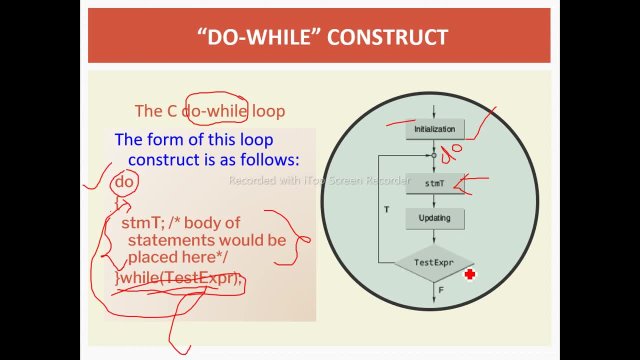 we can increment the value or either we can decrement the value. next is we are checking the test expression. if it is true, the control come to the do while block. it will execute the statement and ye kaptak hoga unless and until that condition become false. if that condition become false, the control come out of the do while loop. 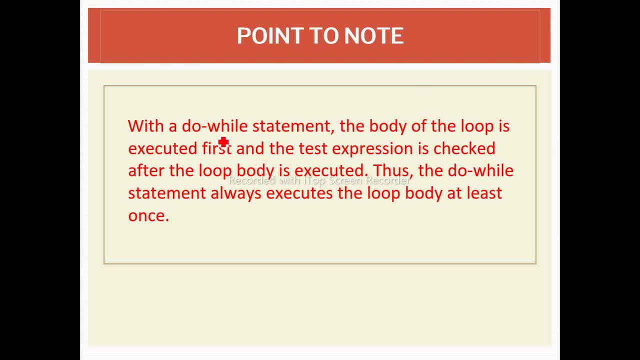 so here the point to note: as do while statement, the body of loop will be the do while statement is executed first and test expression is checked after the loop of the body. that is nothing, but is always executes one loop at least once. ok, so in a do while always executes the loop body, at least. 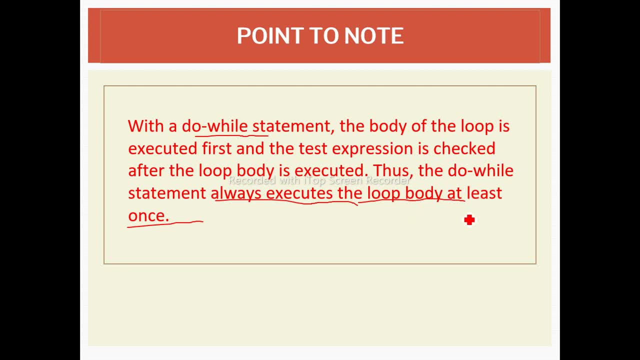 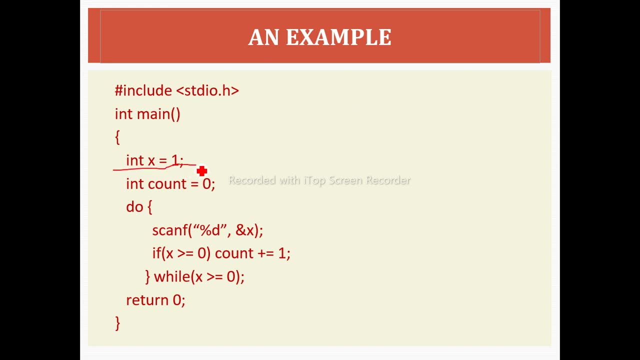 once. ok, so that's why this do, while known as a post test condition. so example is given here. firstly, we will, we are initializing the x to the one. after that we are counting the value again. do, that is, scanning the value of x from the user. if x is greater than equal to zero, we are performing the. 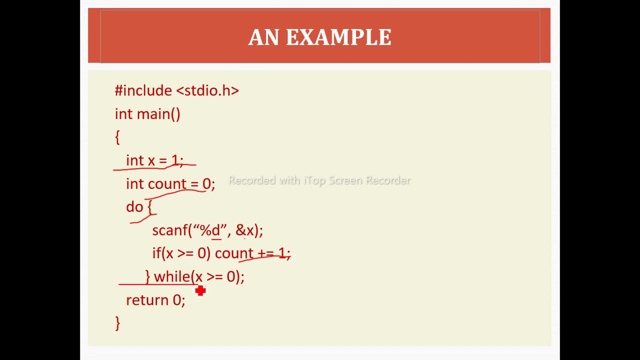 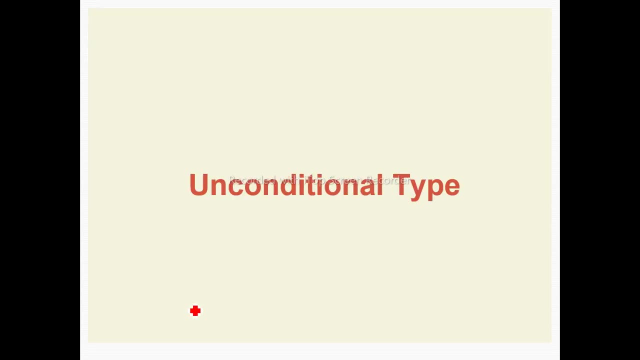 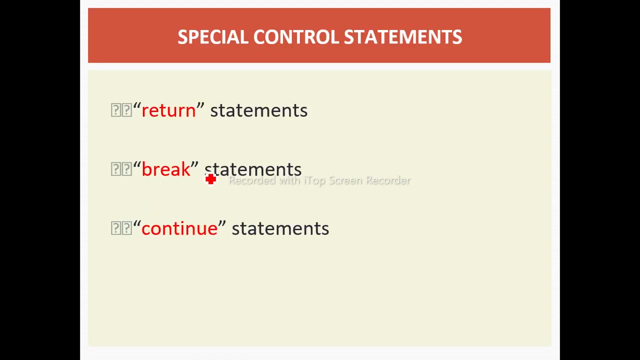 count value and after that, whenever the x becomes greater than equal to zero, we will come out of the loop and we are going to return the value. ok, next is unconditional type. unconditional type is nothing, but here we are not giving any condition, we are just executing our program. so there are three statements: return, break and continue, so out. 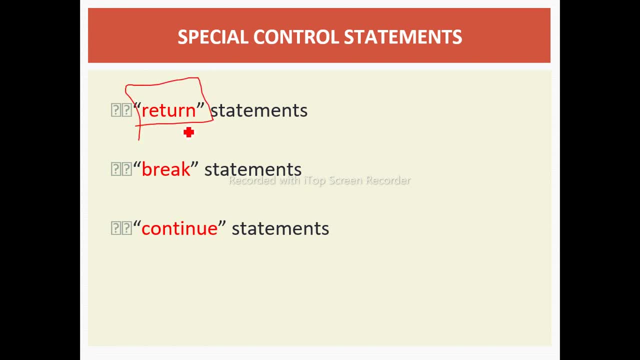 of that return. we have learned the return return is nothing but returning the value of a function. ok, just a main case. out humlo kalik, the return zero. if our main function is not returning any value, we are writing return zero. so return statement is always used with the function. 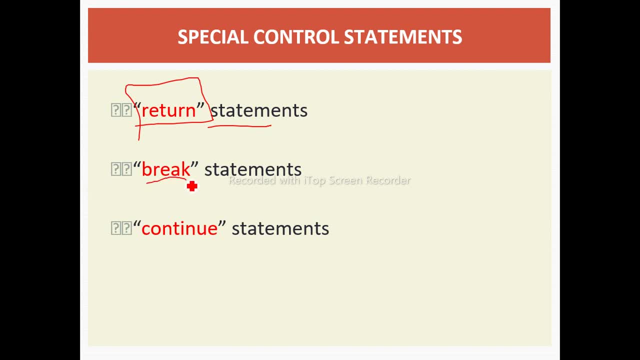 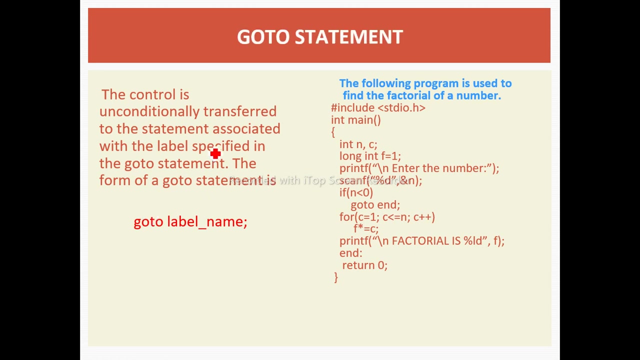 break statement. humho habhi pada break. statement. we are using to break the control sequencing. okay, and where we are using this break in a switch, state me and next continue. continue is used to just continue the program now. next is go to statement. okay, so go to statement. this is the unconditionally transfer. why? because here in a 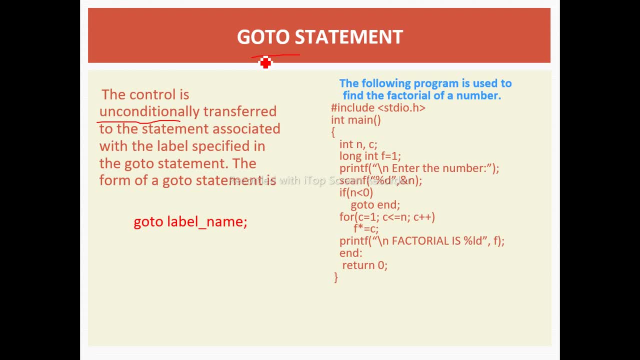 go to statement. we are not checking any of the condition, we are just passing the control to that statement, so so the go to statement unconditionally transfer to the statement associated with the label. go to case. case are used with the label always, so the go to go to is the keyword and label. 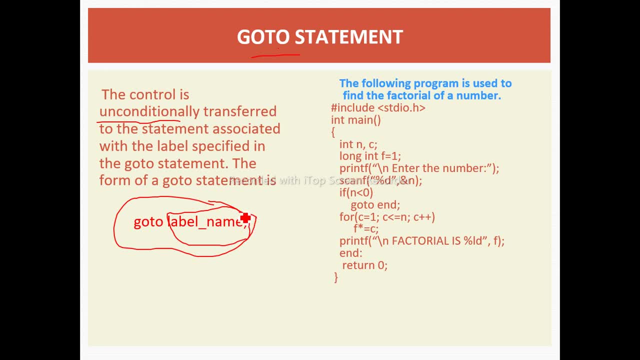 name. so we can give any of the label name, label name, but go to always will work with the label name. so here the example is given. firstly, we have declared the variable. we have initialized the variable by the printf statement. we have displayed the statement, enter the number. 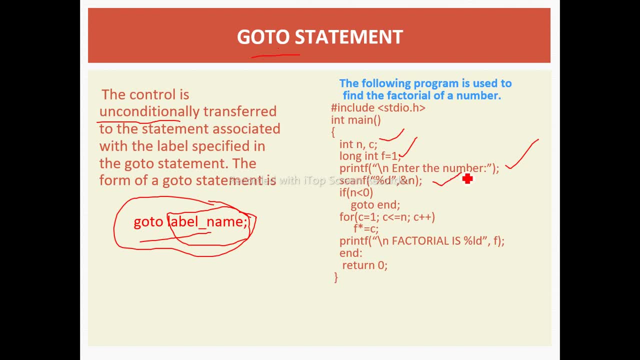 after that we have taken the variable value from the user by using the scanf statement. next in if block, we are checking. if that number is less than zero, the control will get passed to the end. that is go to end. and where is that end here? okay, so again: number less than zero, it will come at the end. 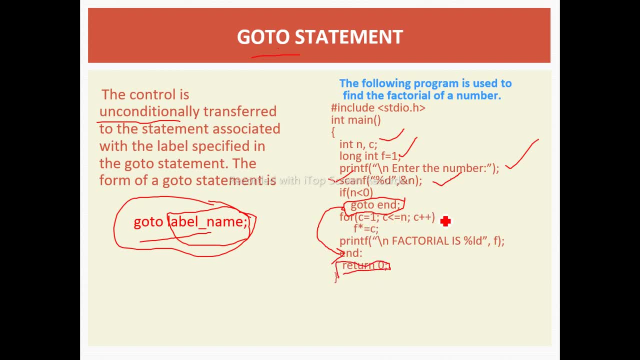 okay, if it is not, it will execute this for loop or flow. for block c is equal to one, it will check whether c is less than equal to n, so it will count this factorial value. that is nothing, but just now we have seen that koi bhi number agar less than zero hai. 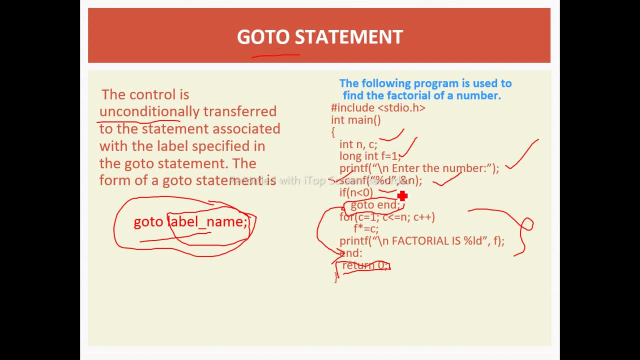 we cannot find the factorial. to find the factorial of a number, that number should be a positive. so here we are checking whether that number is positive or not. if that number is negative, then directly here we are passing the control to the end, that is, by using go to. 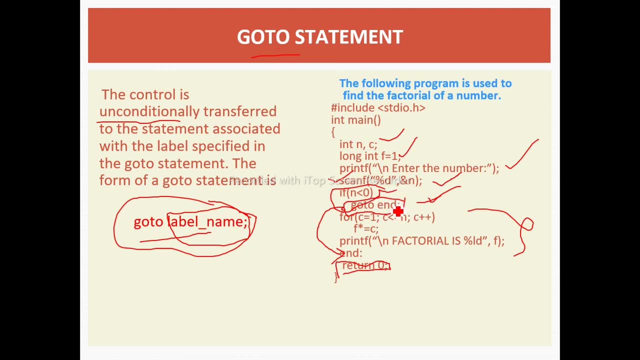 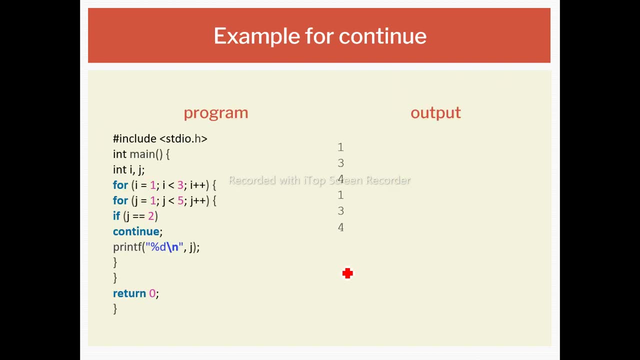 with the label and here what is the name of the label end and where we have written that end at the end of the program. so this is a go to statement. next, example of continue. so example of continue is just used to continue the program. agar condition, agar false bhi aaya hai, then also agar hume program ka flow continue karna hai, then 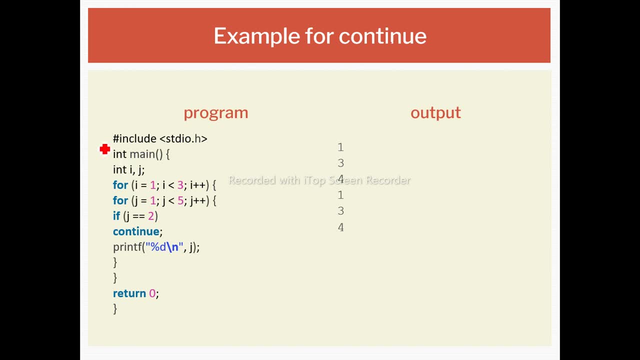 we are using this continue statement here. firstly, we have used the header file, after that the main function. next is here: int i, j, that is, we have initialized, we have declared the two variable and i and j. after that, in that, i and j, we have taken the two for loop. first, for loop will start from the. 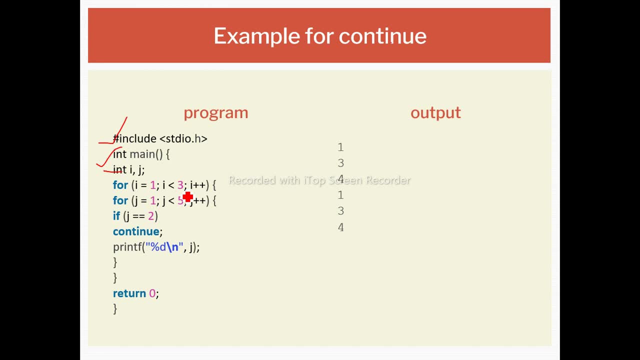 i and it will execute up to the 3 value and within that for loop again, we have taken the another variable, j variable, and the condition is: i is less than 5 and within that, here we are checking if j is equal to equal to 2. 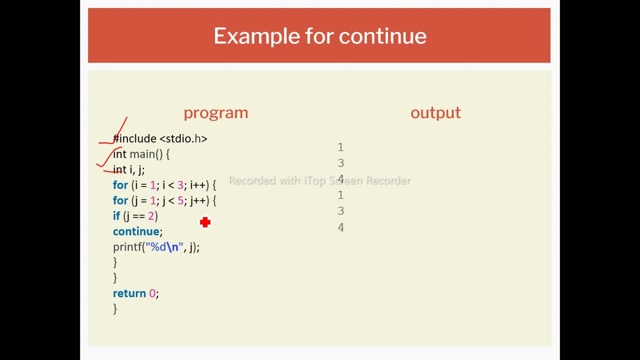 we are again continuing the execution. okay, so i is equal to 1. will get initialized again next. j is equal to 1. okay, and again here we are checking the condition. j is equal to equal to 2. yes, it will continue to print j, so one. so it will print the j value, okay, next. 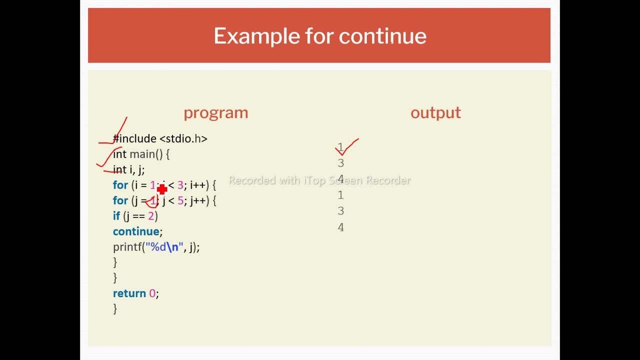 i will get increment one, so this will be 2. so 2 is less than 3. yes, it will come inside the loop. it will execute this for loop once it will check and j will become 2. 2 is less than 5: yes, so j is. 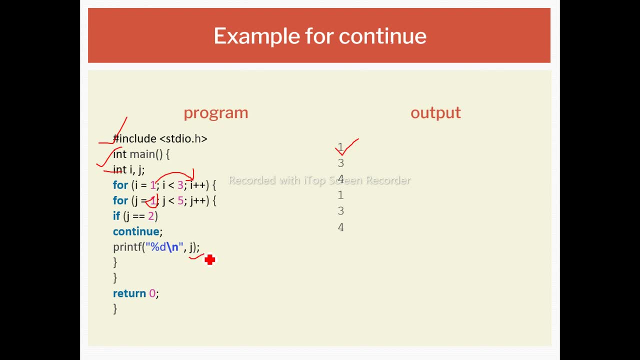 equal to equal to 2. we are printing the value of j again. again, the same form will get executed: 1 3 4. 1 3 4. 1 3 4 in this form why? because always we are printing the j's value. 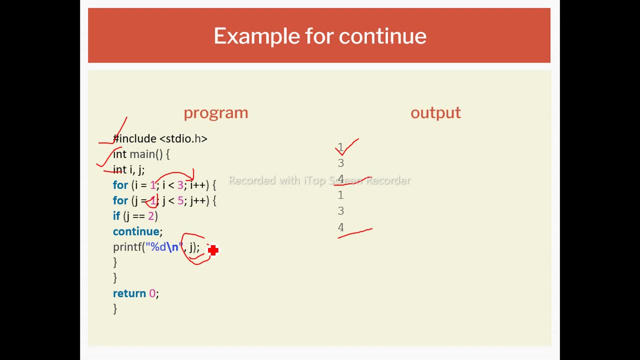 we are not printing the i's value. got this everyone. next is example of break statement. so here, firstly declaration of header file, then declaration of main function, then declaration of variable. here i is equal to 1, i is less than 50. that is, 1 is less than 50. yes, 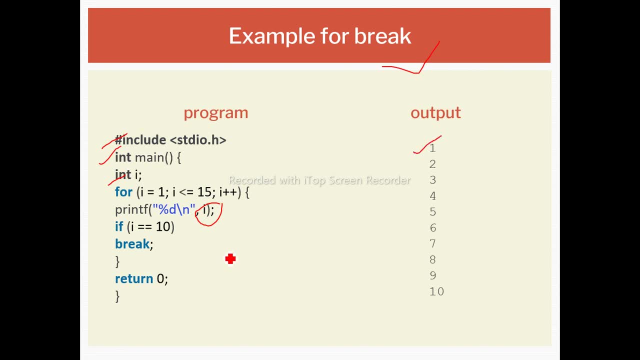 we are printing the 1 value. okay. next again, we are checking that. we are incrementing that. i value i 1. it will become 2, so 2 is less than 15. yes, we are going to display the 2. it will increment by 3. 3 is less than 15. yes, 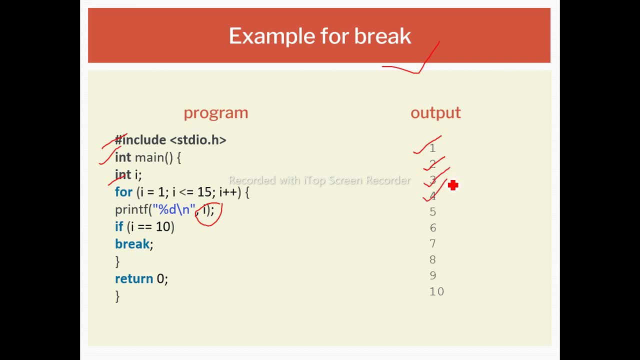 okay. next 3 is uh. next it will become 4. 4 is less than 50 up to the 10, but jabbo 10. huga, it will check that if i is equal to equal to 10.. 10 is equal to equal to 10, it will. 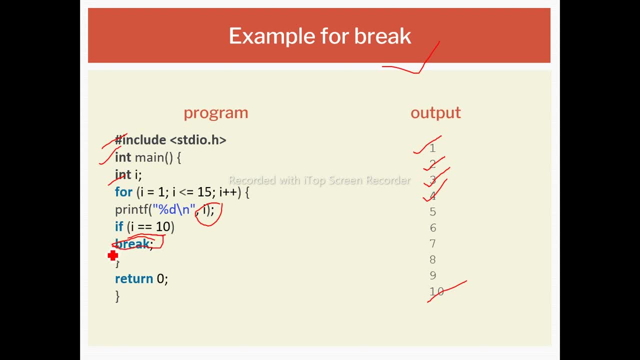 break the control and this come out of this loop. aur wo execute kap tak hoga 10 tak why? because yaha pe agar humne condition di hai less than 50, but yaha pe every time it will check whether it is i is equal to. 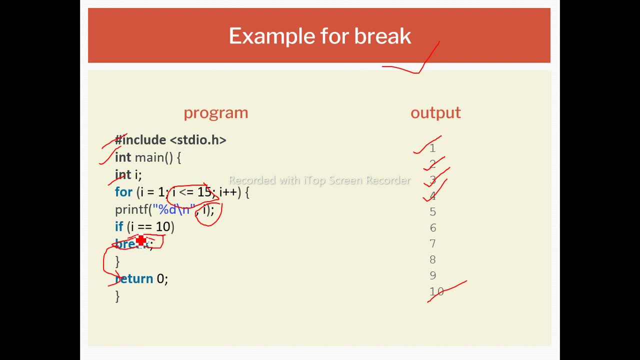 10, so it will compare the i value and when the i value becomes 10 it will come out of the loop and it will exit from the program. so this is the use of break statement and next is go to statement. just now we have seen the 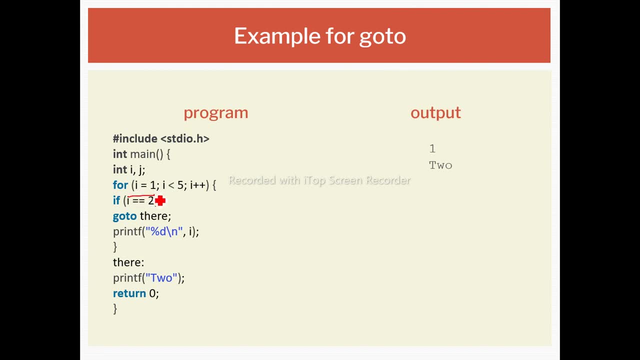 example, i is equal to 1. that is, we have initialized the i value. that is, 1 is less than 5. yes, yaha, pe check hoga. 1 is equal to equal to 2. no, we are incrementing the i value 2. 2 is less than 5. yes. 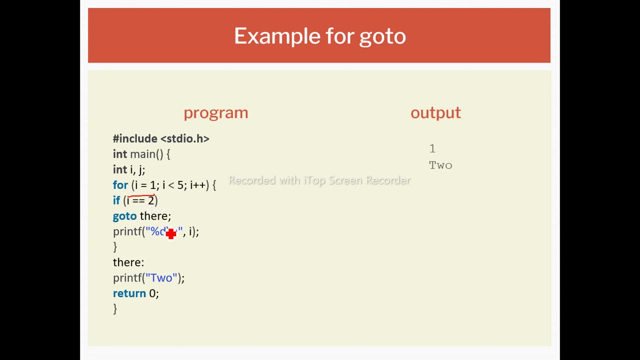 2 is equal to equal to 2. yes, so go to there. so there kaha pe hai the control pass to this there label. so there label ke baad me kya hai print 2, so that's why yaha pe kya print hoga.